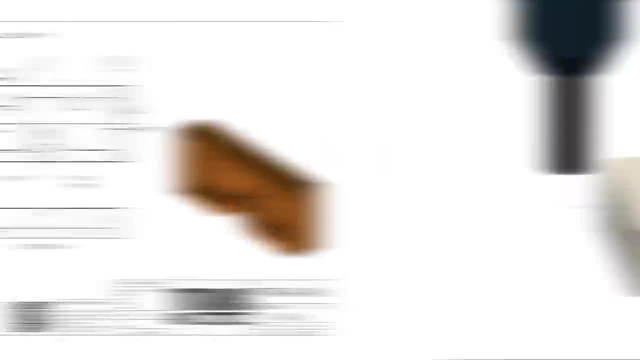 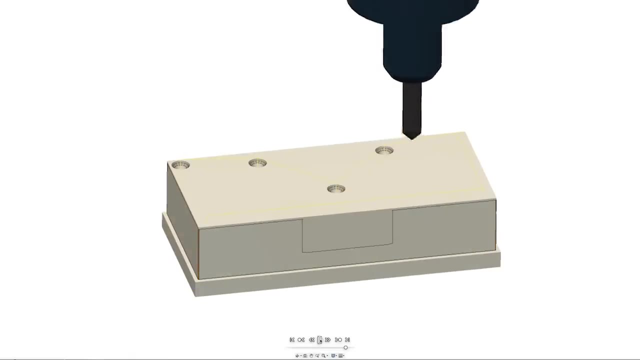 the pockets and shows the part complete. So let's actually profile the part with a half inch end mill and come back and actually chamfer drill and tap the 1032 threads. One thing I'll also say is G and M codes. So let's actually profile the part with a half inch end mill and come back and actually chamfer drill and tap the 1032 threads. One thing I'll also say is G and M codes. So let's actually profile the part with a half inch end mill and come back and actually chamfer drill and tap the 1032 threads. One thing I'll also say is G and M codes. 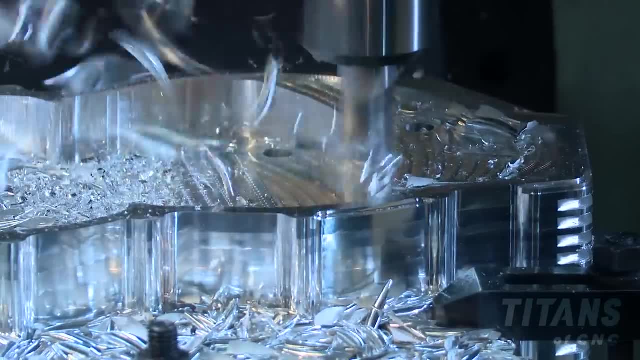 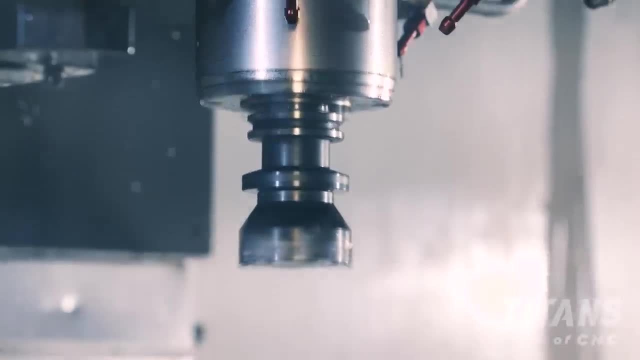 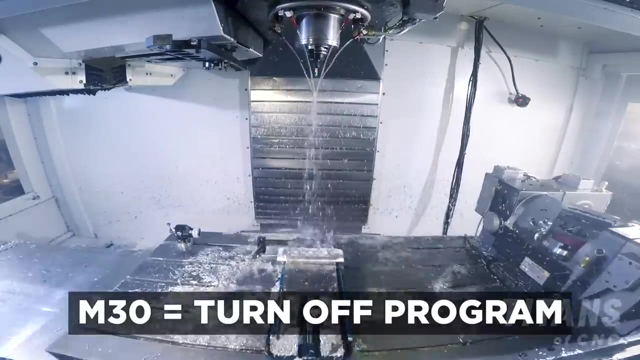 What are they? G codes actually create action. It makes the machines move. M codes usually turn things on or off. So to turn on the spindle you'd hit M3, spindle turns on. Turn on the coolant- M8, shut off the program- M30, stop a sub- M99, and on and on. 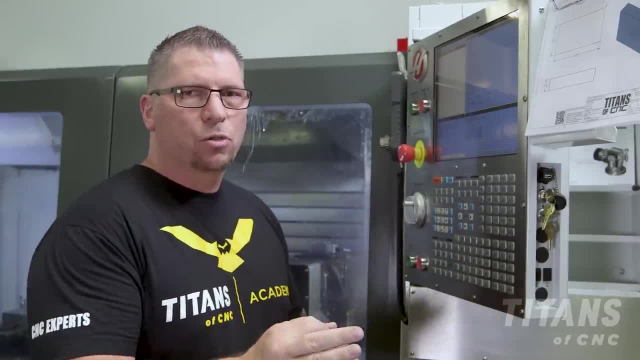 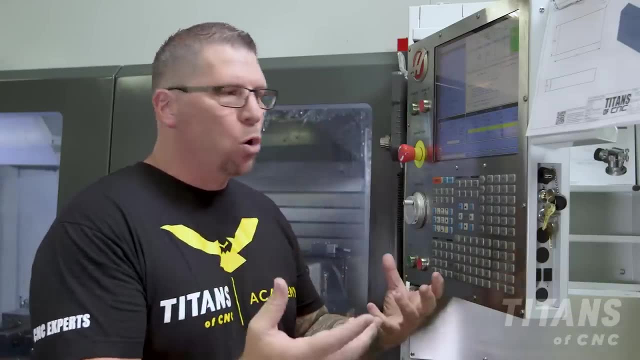 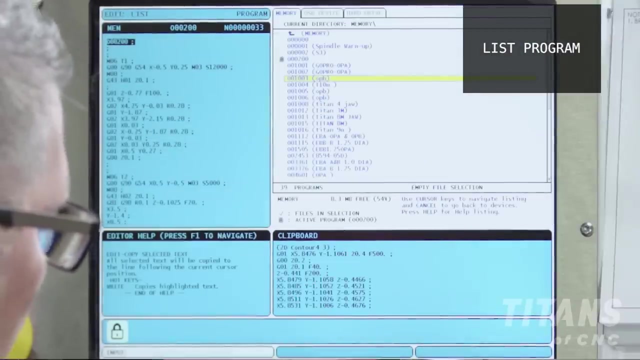 So G codes create movement, M codes turn things off and turn things on. So now the first step in programming is to actually create a program. To create the program, I'm going to hit list program. I'm going to hit O. All programs start with the letter O, So I'm going to hit O. 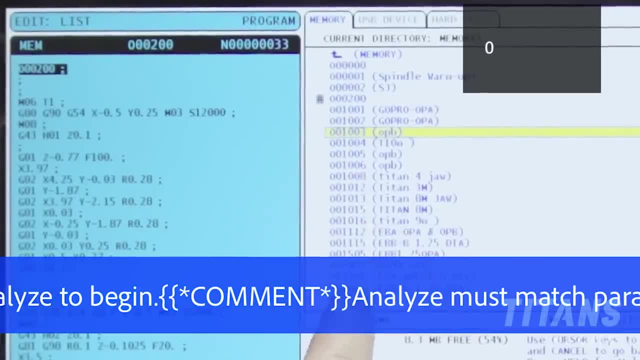 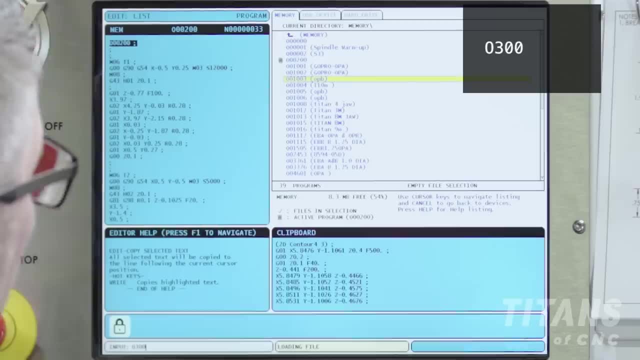 I'm going to look up and see the different programs in there and pick a number that's not being used, And I'll pick 300.. I'm simply going to hit enter And boom, there it is. From that point I hit memory. 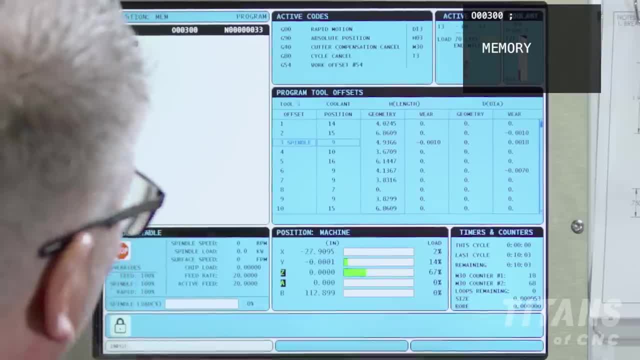 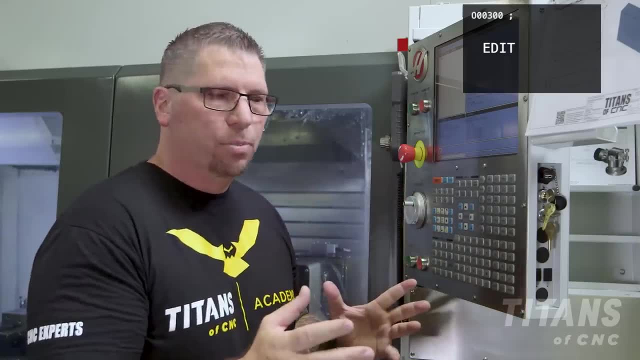 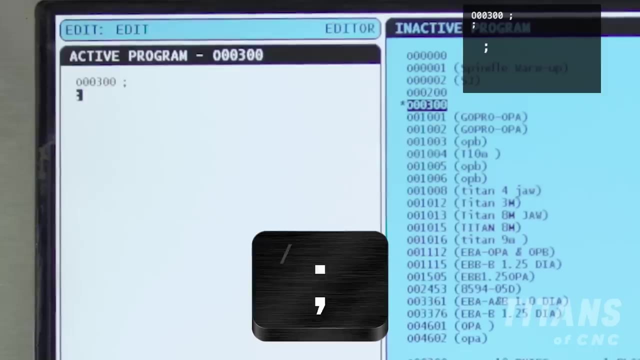 Boom, It sets over. here. I hit edit, I'm able to toggle around and actually create my program. So the first thing I'm going to do is create some space. This end the block key right here is genius. so I like just kind of hitting it. Boom, Boom, Creating some space, Getting away from the top. 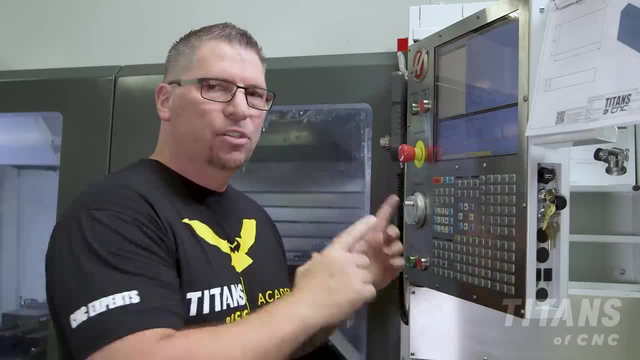 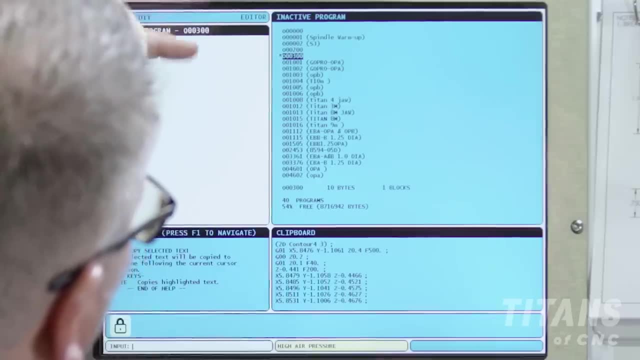 This is where I can write instructions. XY zero is upper left, Z zero is top. Move in, Do this, Do that. These are the tools- tools that all be right up there in my header Now to program these different tool paths, I'm 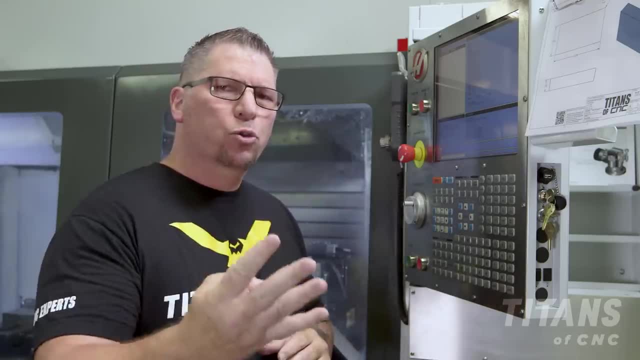 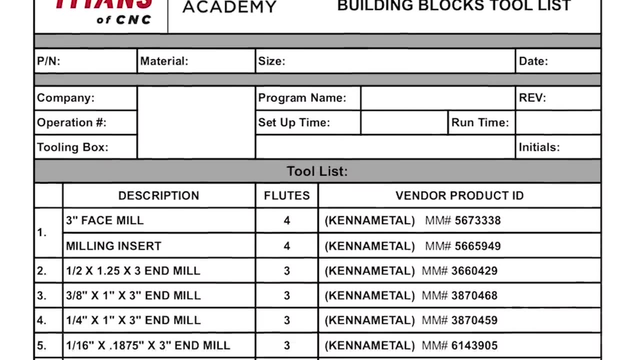 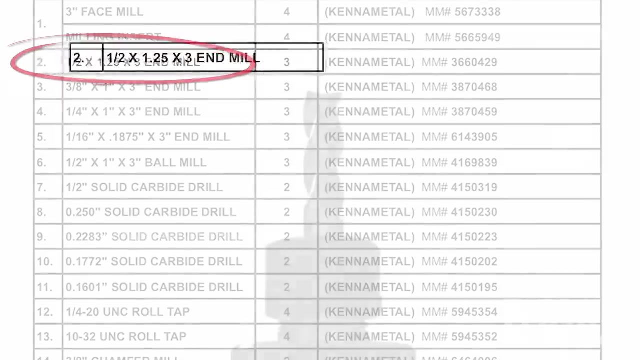 going to actually use four different tools and I'm going to pull those tools off of the building blocks tool list. It's a standardized tool list of 16 tools that allows you to make all of the building blocks. So the first tool is tool number two. It's a half inch end mill and we're going to 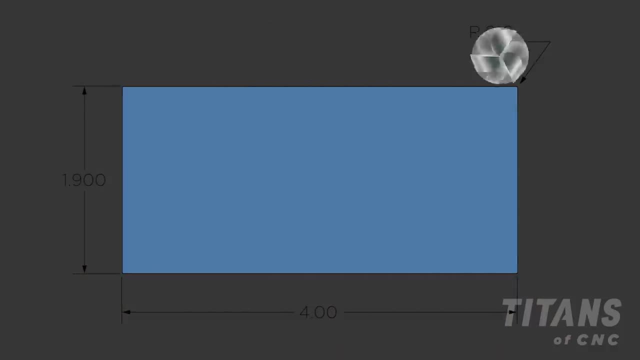 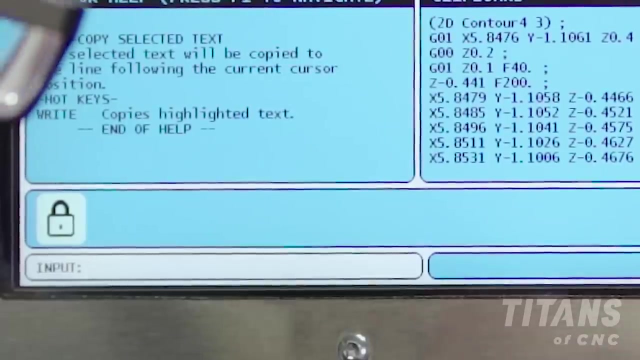 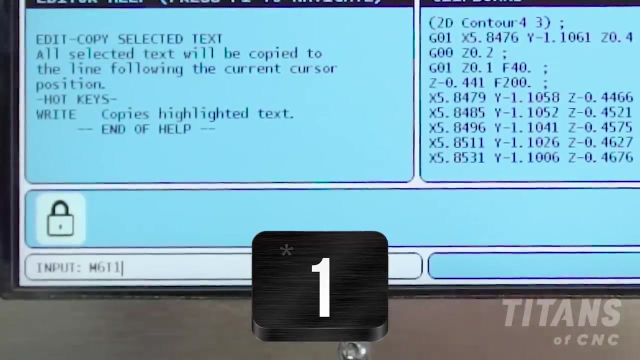 use that half inch end mill to actually profile around this part right here. All right, so now let's actually write this program. So the first thing we're going to do is we're going to hit M6.. Go grab a tool, Let's do tool one, and then I'm going to hit end of block enter. 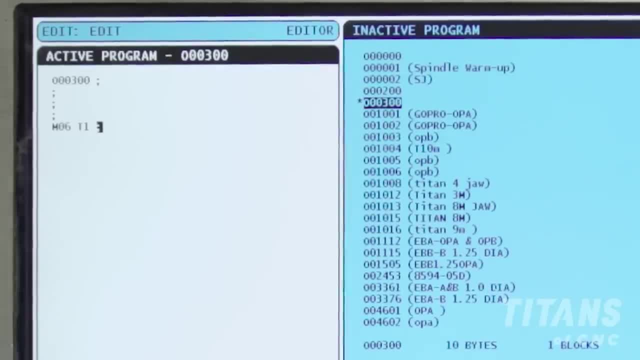 M6T1.. You see the zero. If you hit M6, the machine will automatically put the zero in. You don't have to hit M6T1.. You see the zero. If you hit M6, the machine will automatically put the zero in. You don't have to hit M6T1. 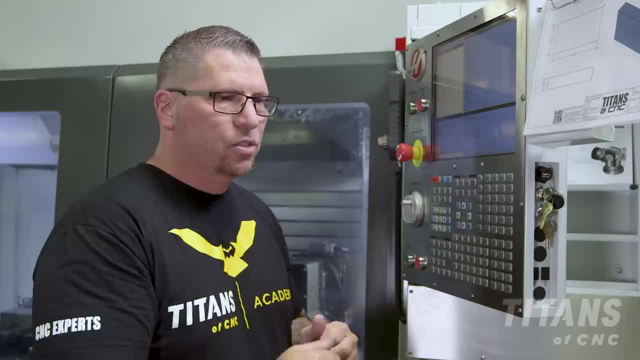 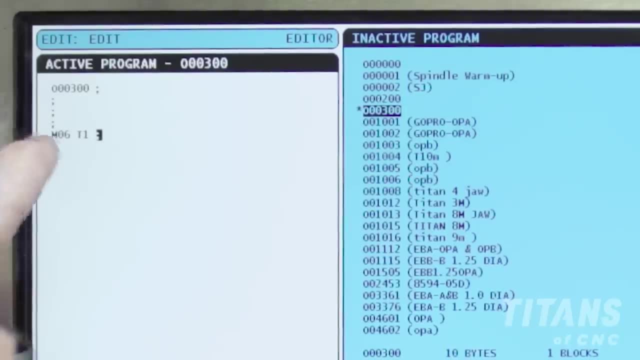 hit M06.. Just hit M6,, T1,, end the block, enter or just enter and the zero will automatically appear. So this is telling the machine to go get tool number one, which is our half inch end mill. Next thing we're going to do is we're going to go to location, So we're going to say XY0 is in. 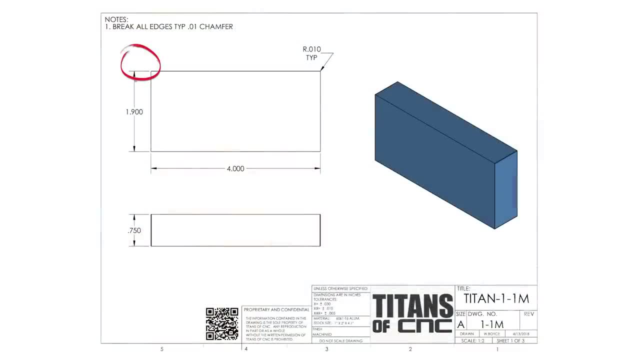 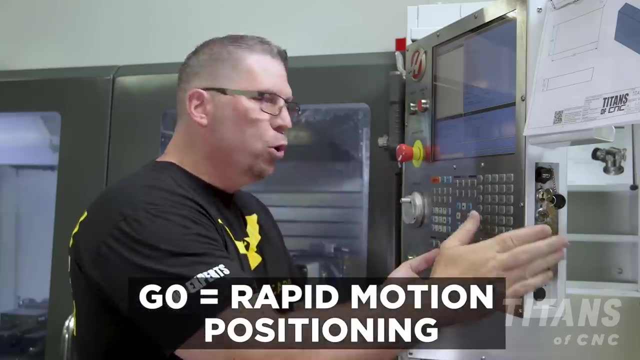 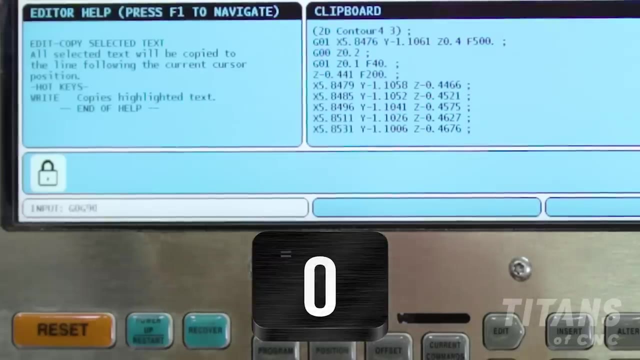 the upper left, so right up in this corner, right here. All right, so now that we have our tool, we're going to actually go in. We're going to say G0, rapid movement: Move as fast as you can with no feed rate. Let's get to position. Then we're going to hit G90.. It's just a safety code. 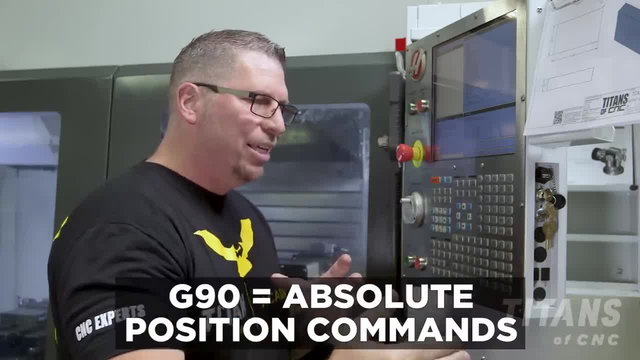 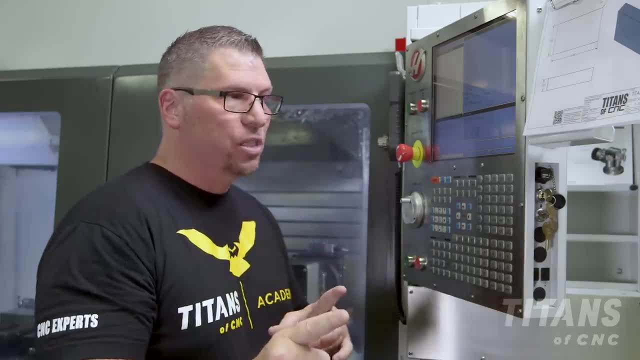 that I like, because some people go into G91 and cancel G91, which is incremental with a G90. And since a G91 can be dangerous, I just like having a G90 at the start of my tool, just to be safe. 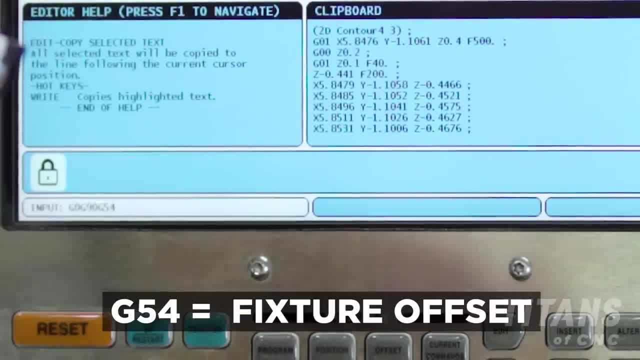 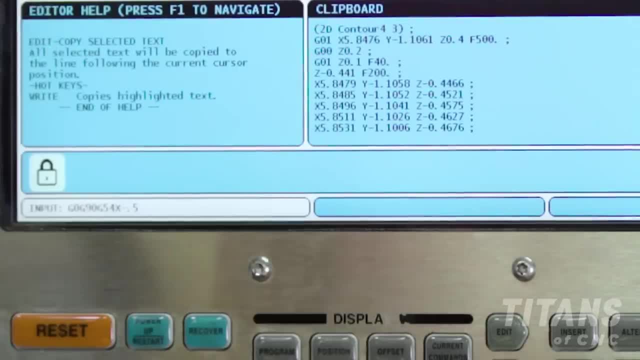 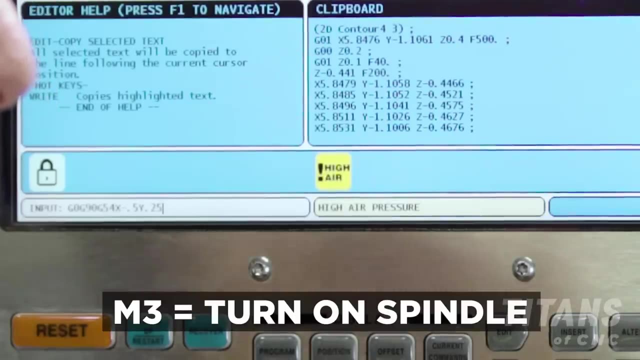 I'm going to hit G54.. That's our fixture offset for that particular part. I'm going to go X negative 0.5, Y 0.25, and then I'm going to turn on my spindle. Turning on the spindle is M3, and then S. 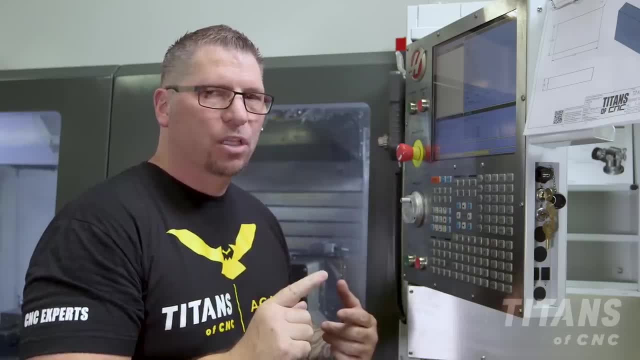 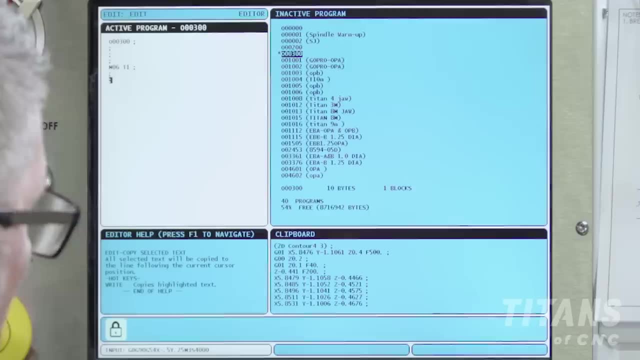 with the amount of RPMs for how fast you want to actually run that spindle. So I'm going to hit M3, speed 4, 0, 0, 0.. And then watch, I'm just going to press Enter. Boom, it's up there with my end of block. 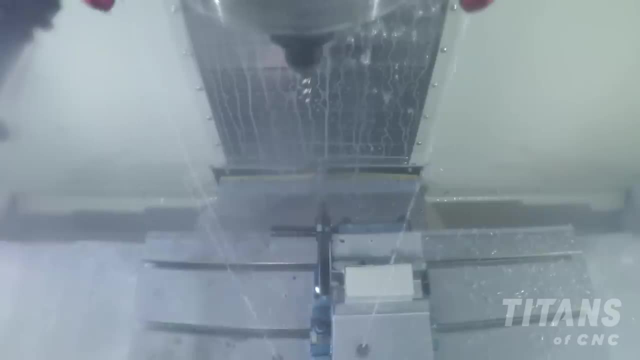 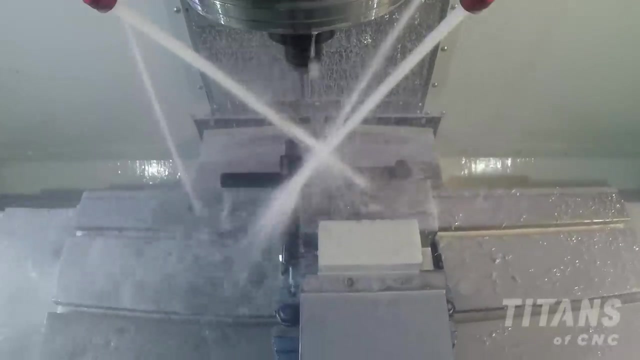 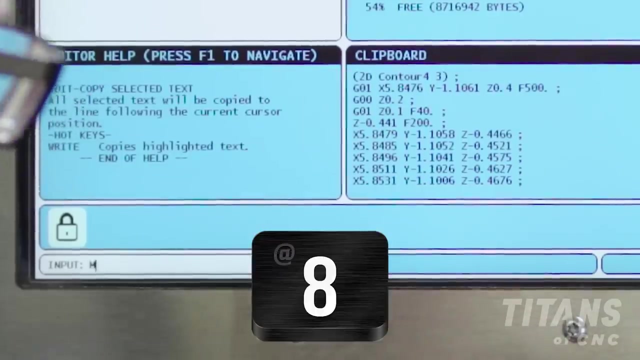 So, now that we're in location, what do we do next? Let's turn on the coolant while the machine is still up here, so that if there's chips in the line, they have a chance to flush out. So once the tool engages the material, you'll be blasting that coolant. So I'm going to turn on M8, coolant. 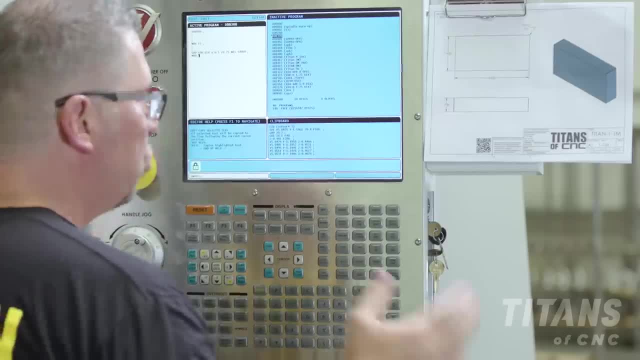 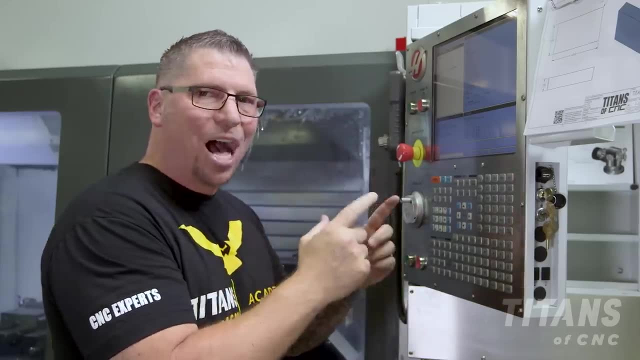 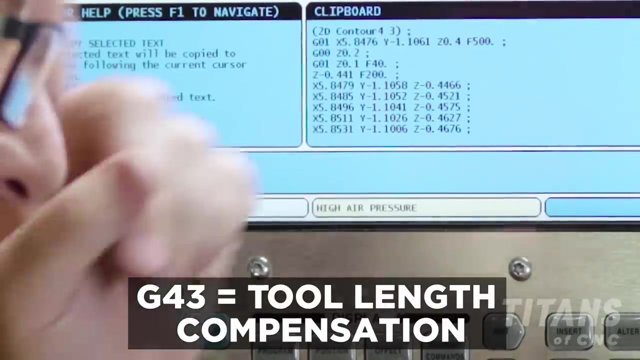 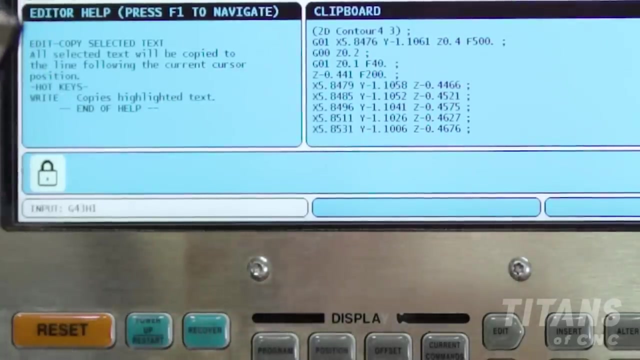 on Enter. All right, Now the machine is reacting off of It's home positions, But I want it to react off of the height offsets that we got when we zeroed off our tools. So how do we do that? G43, go read height offset H1 for tool 1, height 1, H1,. 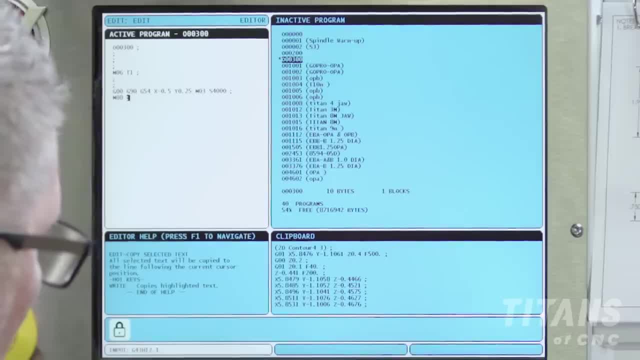 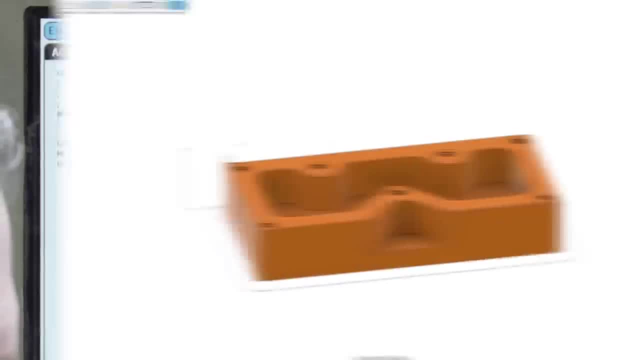 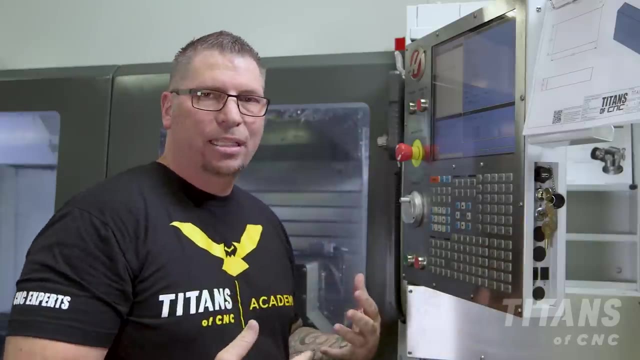 and then Z, point 1, and then Enter: Boom. So all of a sudden it reads the offset. Now it knows where the material is, And then it drops down 100,000 shy of that surface. Now I just like creating a. 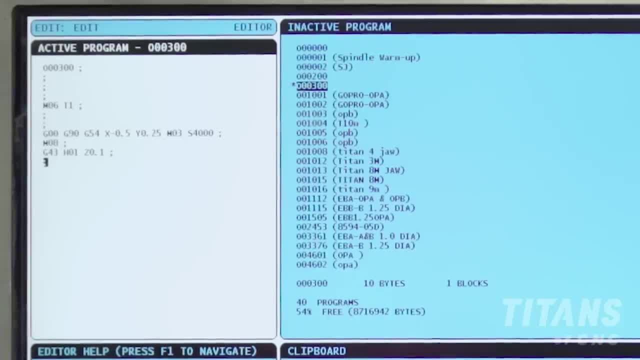 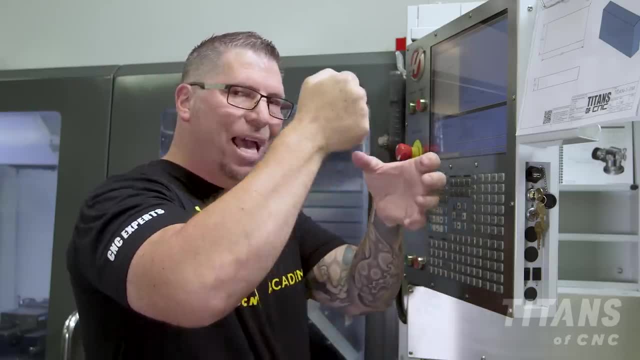 little bit of space. So I'm going to create a little space pop in an end of block right there. So when we're above we can rapid G0. We can move around. We're not going to hit anything. But now we're going to actually submerge, We're going to drop down and engage the material. So 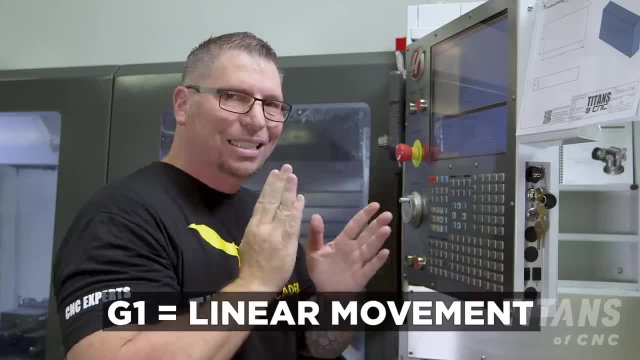 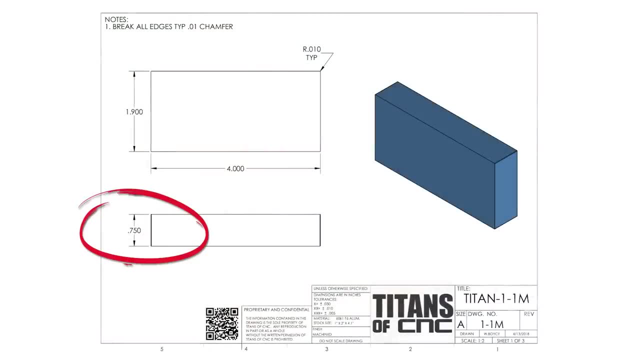 I'm going to go from a G0 to a G1.. A G1 is a linear movement with a feed rate. My part is 750 thick, So I'm going to drop to Z negative 760.. So I'm going to hit G1,. 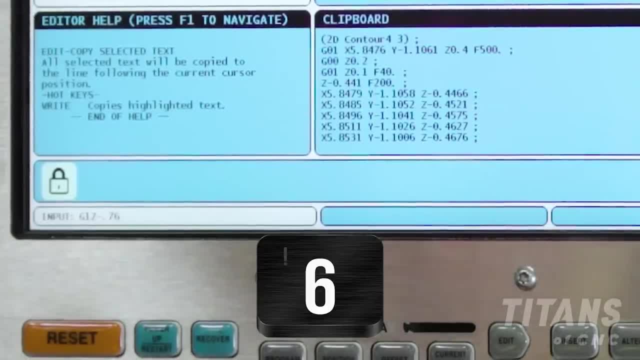 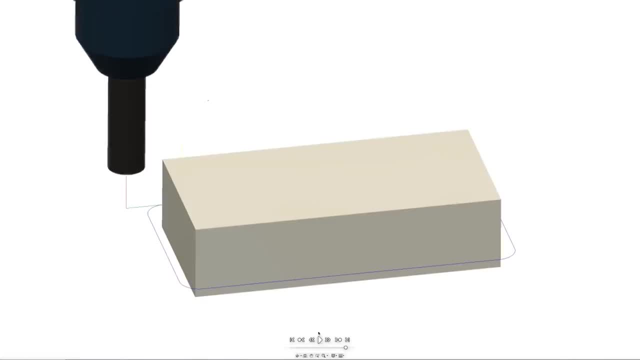 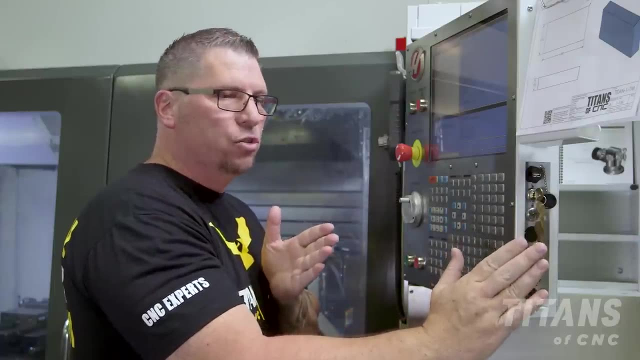 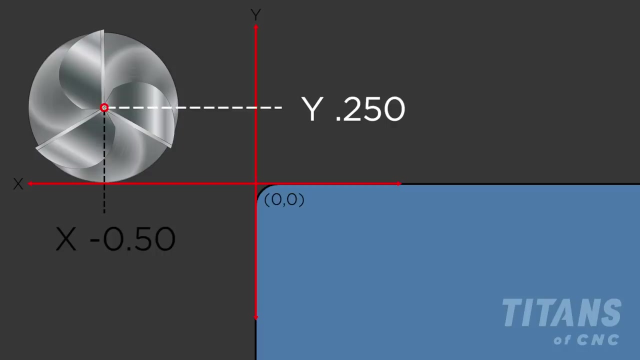 Z negative point 760,, feed 50,, Enter and I'm down. Next thing I'm going to do is shoot across the back surface of the part. So my XY zero is in the upper left. I'm at X negative 0.5.. I'm at 250 off the part because it's center of the tool. So the tool is: 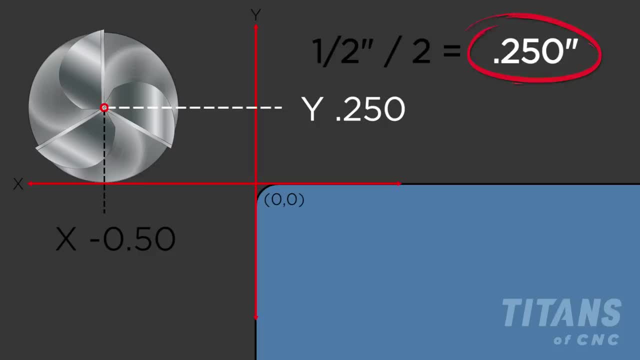 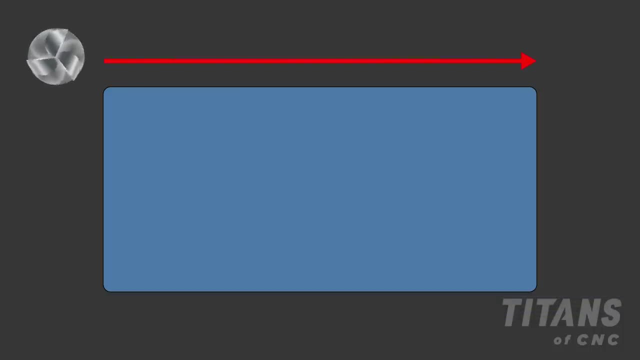 a half an inch, So half of the tool is 0.250. And that's why I have 0.250 right there. Now, as I actually wrap it across here, I got to remember there is a radius corner and it's 10,000.. So what I want to do is I actually want to run all the way across that back end and then 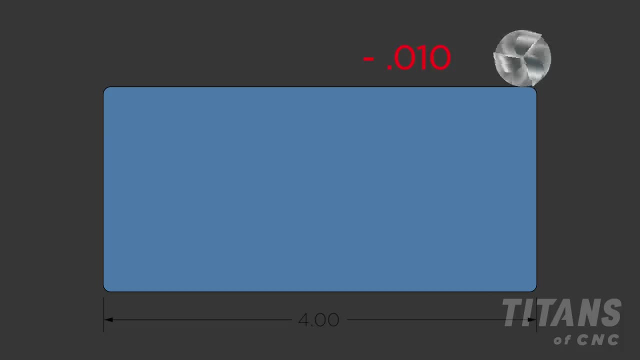 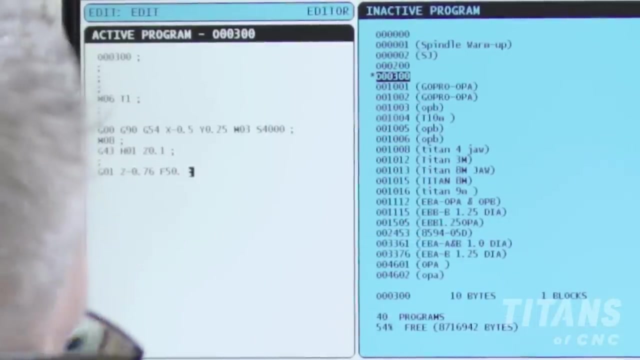 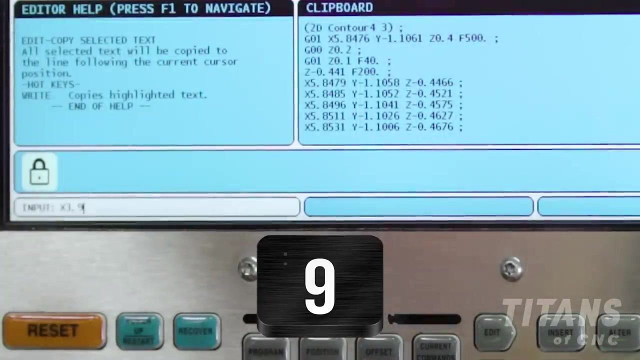 stop 10,000 shy From the end of the part. the part is four inches long. Once we're in G1, if the next line is G1 also, you do not have to repeat it. All I'm going to do is go to location, So I'm going to hit X 3.99. 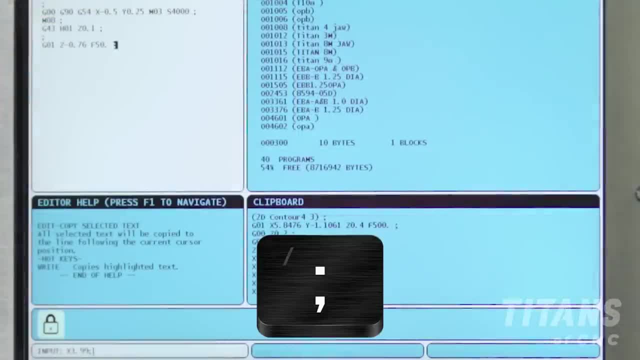 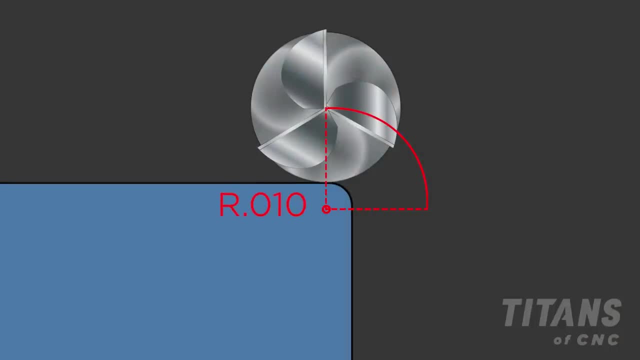 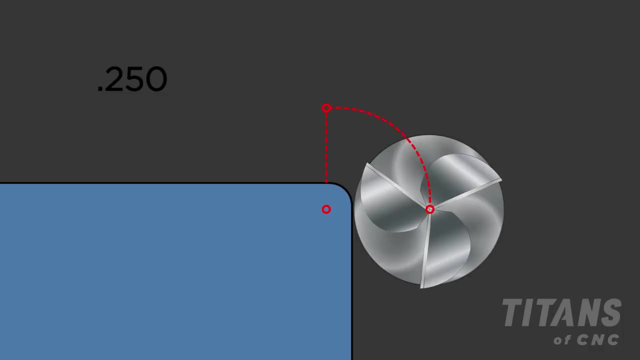 I'm going to leave my feed rate alone and I'm just going to hit Enter. Now we're going to make that radius, so it's 10,000.. So you're always thinking center of the. so, since the tool is 250 and it's going around the radius and the center of the radius is ten. 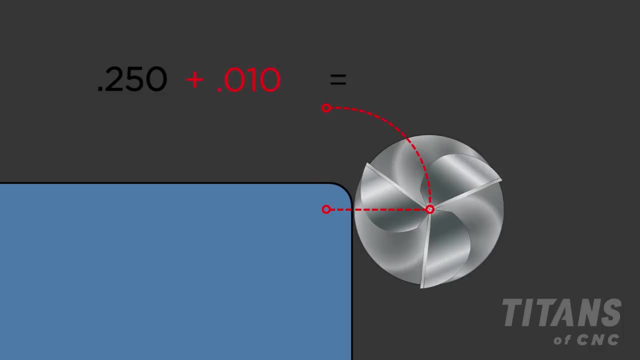 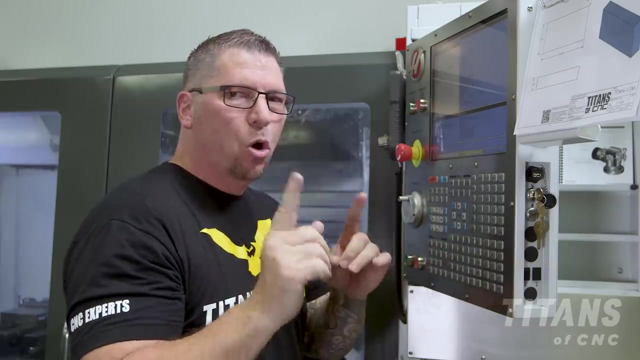 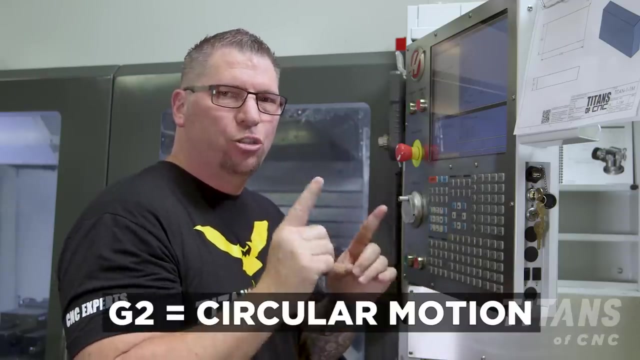 thousandths in, we combine the two and we come up with 0.260. so now we're actually going to radius around it. so the code is going to change. so the radius around it. since we're going clockwise, the code will be a g2, counterclockwise would be a g3. so i'm going to hit g2, i'm going to. 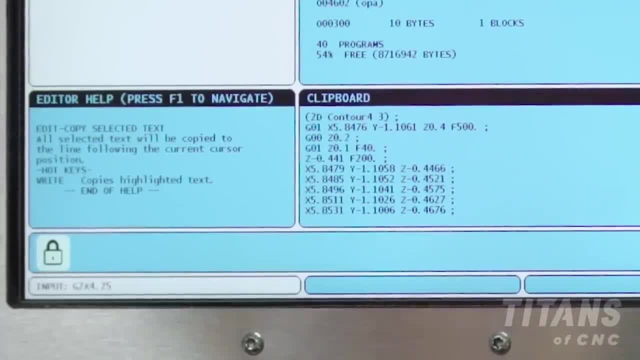 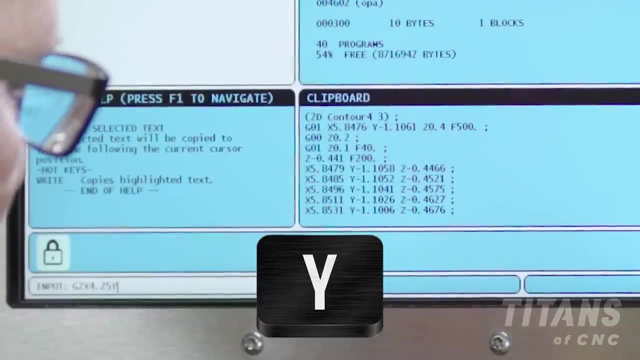 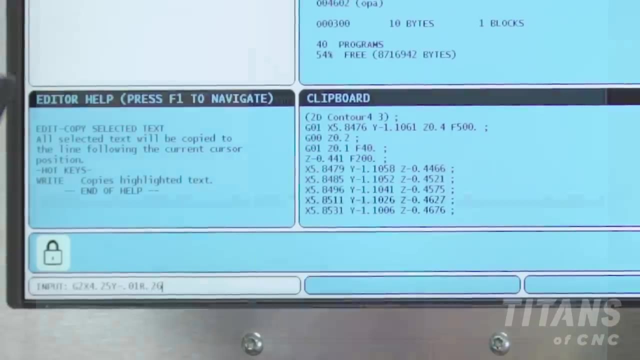 x 4.25, and that's where i'm going to end. i'm going to end at the bottom of the radius, so i'm going to hit y negative 0.01 and then i'm going to hit r 0.26. i'm going to hit enter. 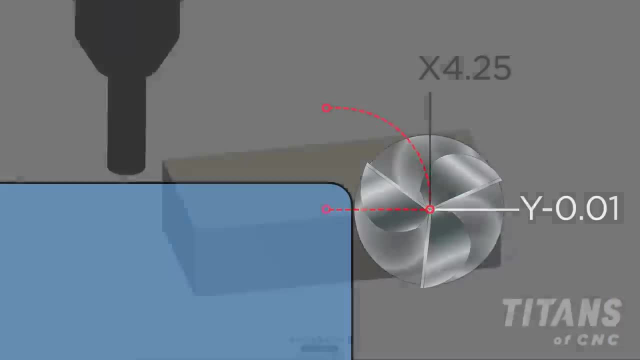 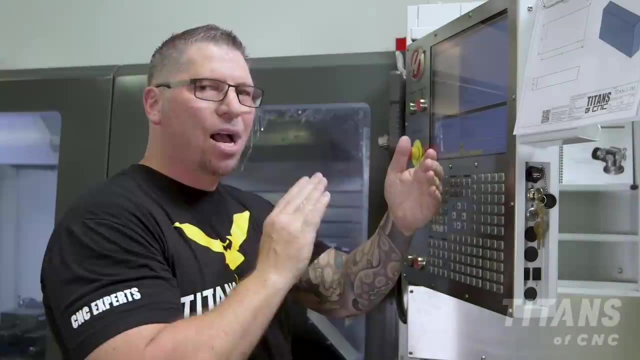 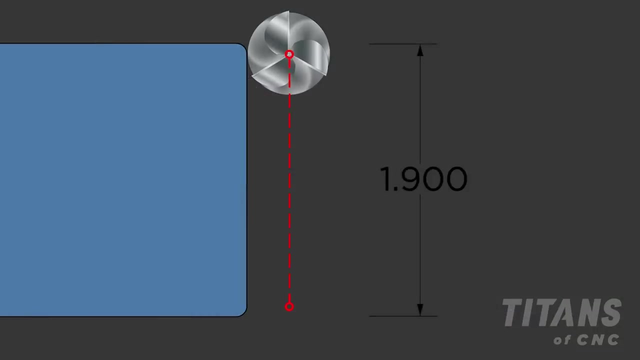 and boom, there you go. and now, basically, i went across the back, i took that corner, i made the radius and now i'm just going to repeat the process, looking at the dimensions on the print. so now i got to drop down. this is 1.9 and i'm going to stay 10 000 shy. so i'm going to drop down in y to 1.890. 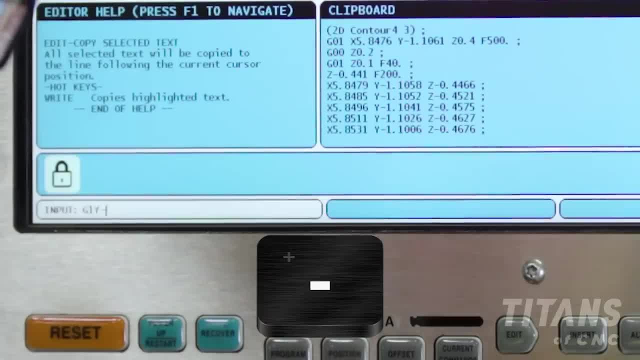 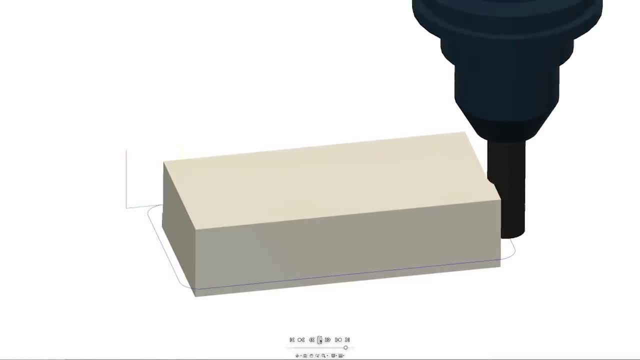 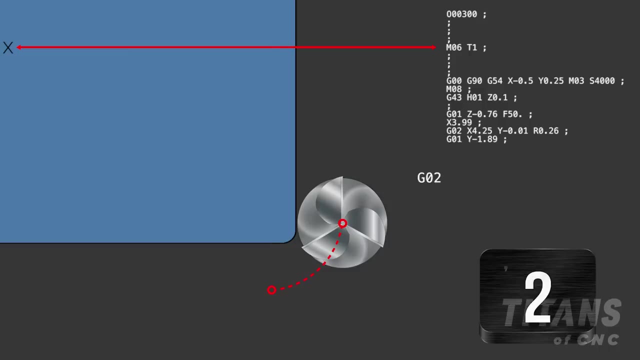 so back to g1. y negative eight nine enter same thing. now i'm coming around the bottom end. so i'm going to go g2 x 3.99, 10 000 shy- now i'm on the bottom- and then y negative 2.15, which is the 1.9 plus the 0.25. 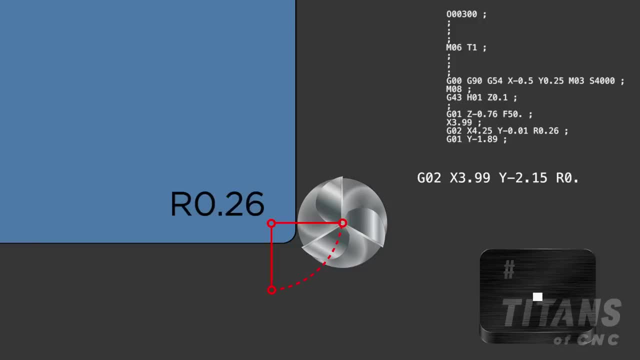 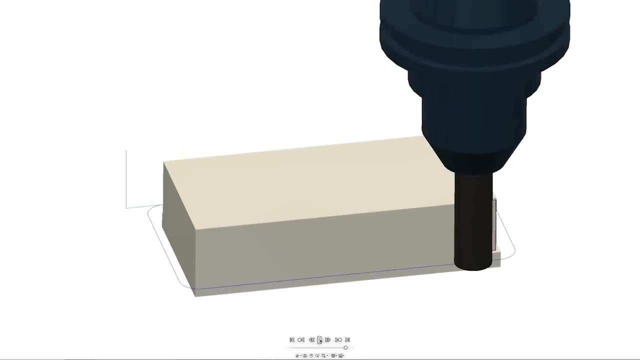 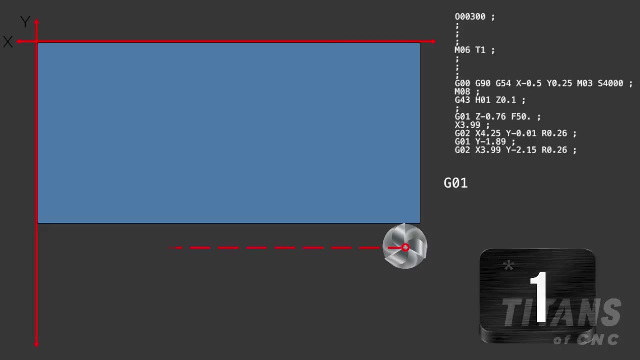 0 and then a radius of 0.26- boom. so now i've taken that turn on the bottom. now i go back to x, 0 over here. so i'm going to go g1, x, point 0, 1. boom, i'm right there. 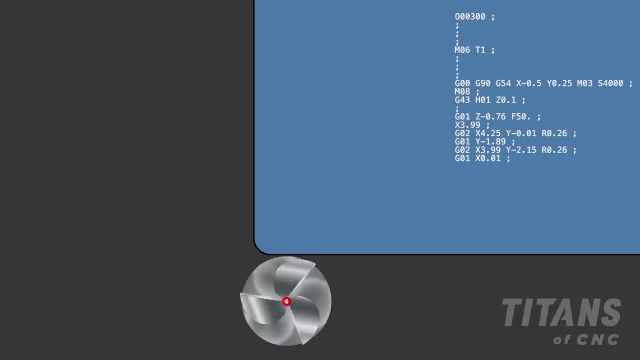 i'm going to take the corner down here. do the same g2 coming around that end, ending at 1.890.. So I go: G2, X negative 0.250, and then Y negative 1.89, with a radius of 0.26. 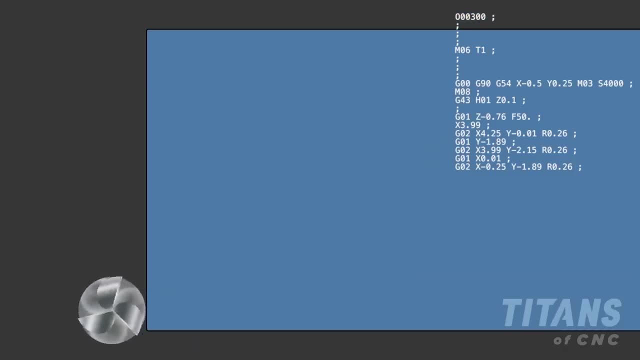 Enter. Now I got to go back to home, back to XY zero, So I'm going to come over here, I'm going to shoot up by just hitting G1, Y negative 0.01.. Enter. And now I'm right here. Why do I not move? 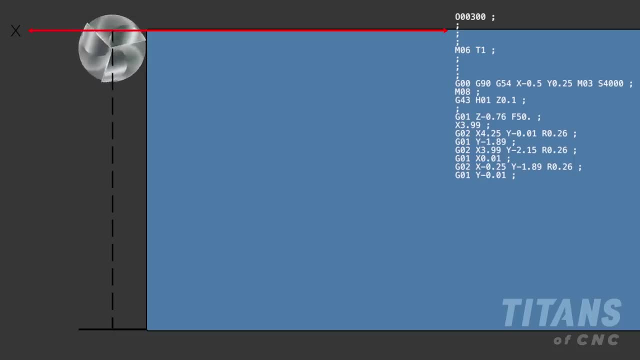 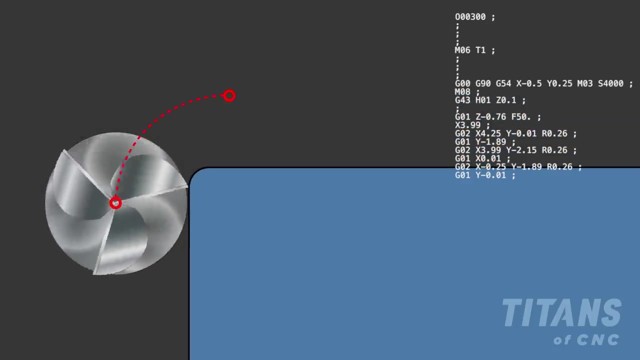 the X Because the X is already in position. So if I just move the Y and the X is in position, the Y is just going to move up and the X is going to stay exactly the same. That's why you see me only changing the Y. So now let's take the turn up here. 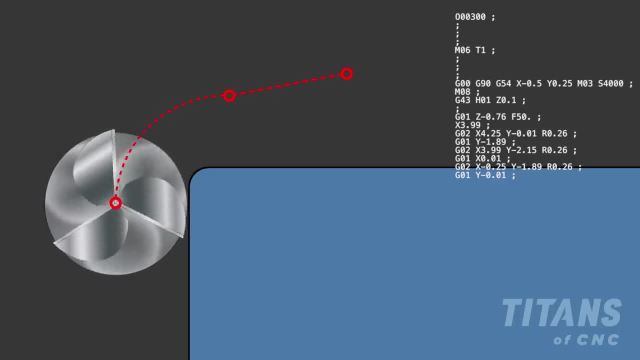 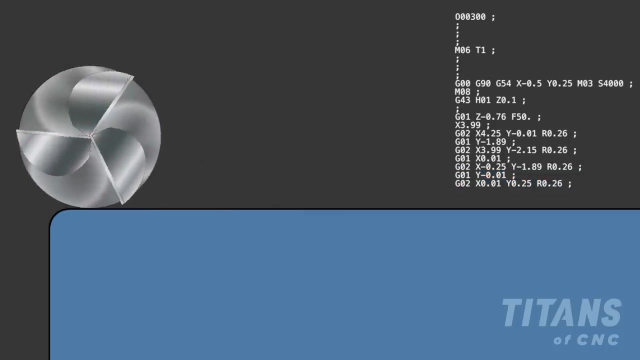 And then I'm going to ramp off it so we don't leave a line, And then I'm going to bring the tool up, So G2, X- 0.01, Y- 0.25, radius 0.260.. Enter, Boom, Now I'm at the top, The top. 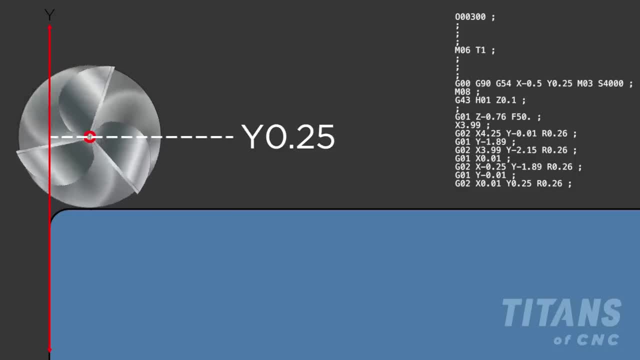 if my Y was at 250, I'd be right on that surface. So I'm actually going to ramp off it. So I'm going to actually move over an X, but I'm going to lift my Y off the surface So it just gradually ramps off the material. 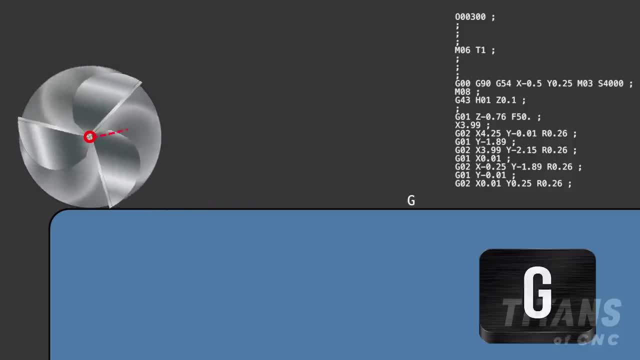 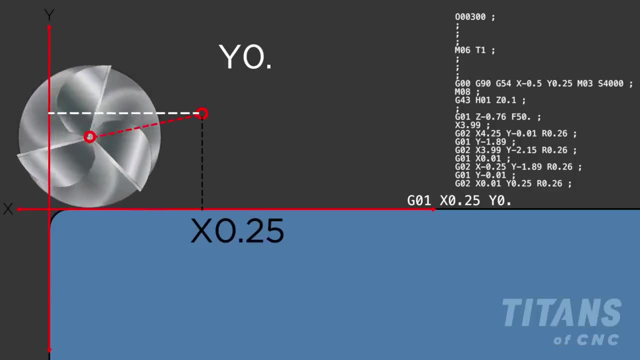 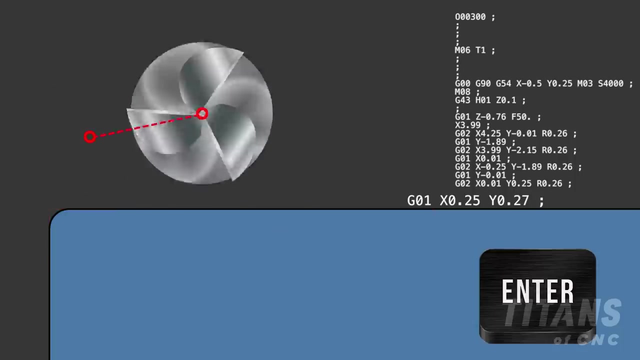 so we don't leave a line. So I'm going to go G1, X, 0.25, Y, point It would be 2.5, but I'm going to go a little bit extra, So 0.27.. I'm going to hit, end the block, Boom. 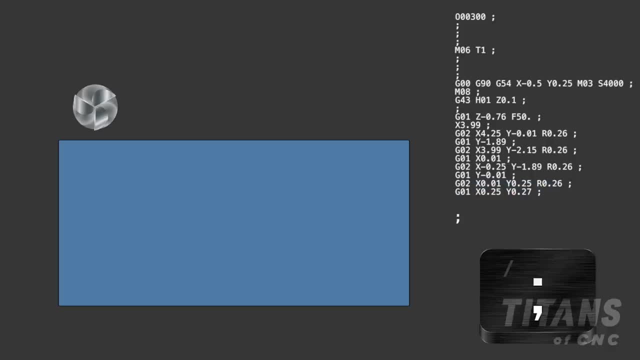 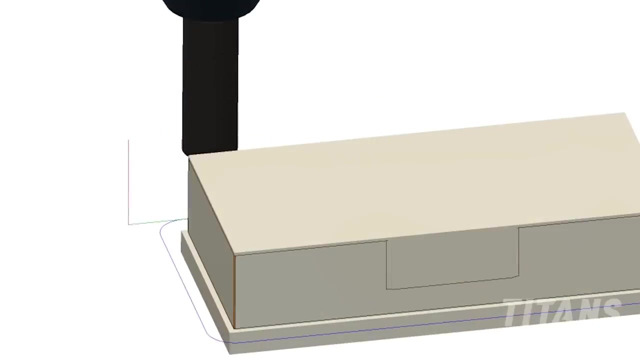 It's right there, Then I'm going to hit end the block. one more time: G0, Z 0.1, end the block. Enter Boom. There you go. So that's tool one Dropping down over here walking around the part doing all the radiuses. 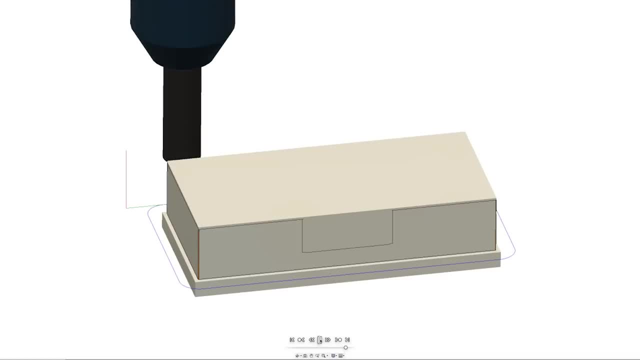 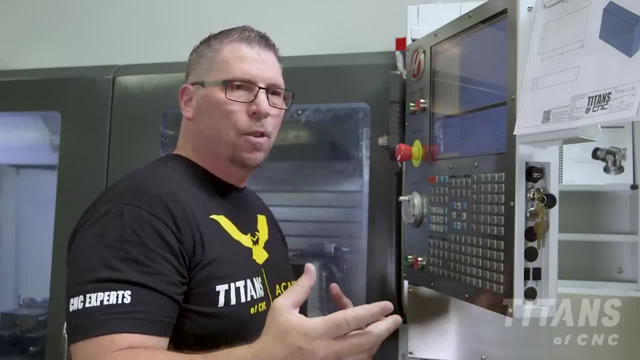 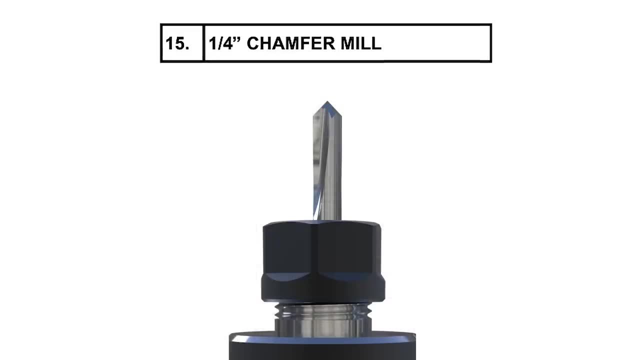 So this is actually going to be pretty easy. Okay, So we're going to use a can cycle and we're going to use three tools from the building blocks tool list. Okay, So we're going to start with the quarter inch chamfer tool, number 15.. Then we're going to go to the 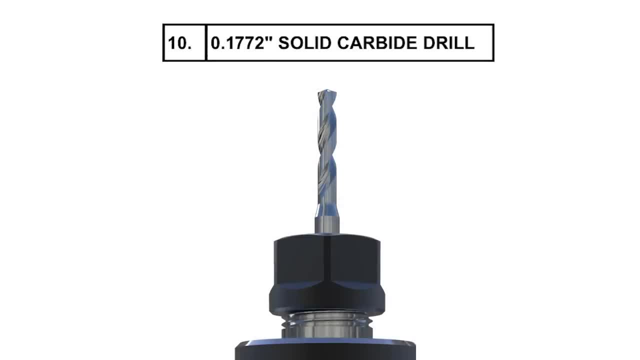 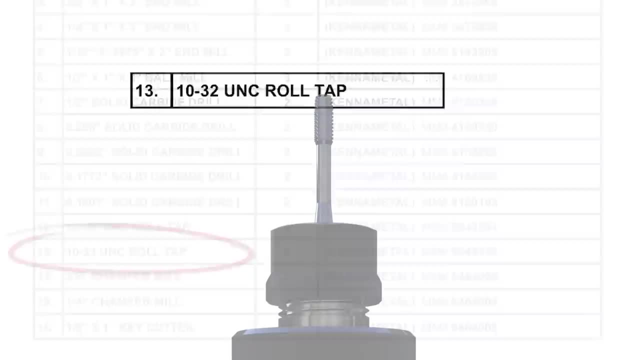 177 drill, which is the proper drill size for a roll tap for a 1032 thread. And then we're going to finish it off with a 1032 tap, And then I'm going to show you a trick to make it quick. 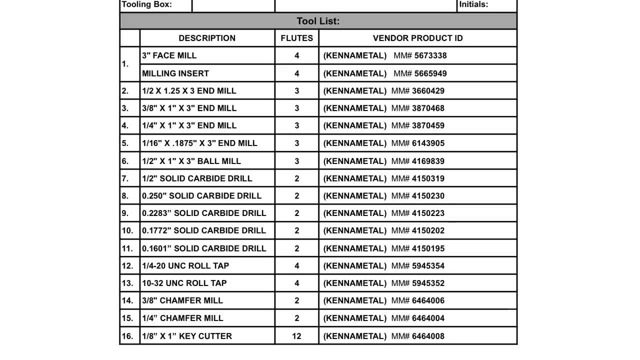 and simple and precise. So the tools are standardized, but I'm actually going to change them. I'm going to change them to a 1032 tap, And then I'm going to change them to a 1032 tap, And then I'm going to change them to a 1032 tap, And then I'm going to change the order. So we're. 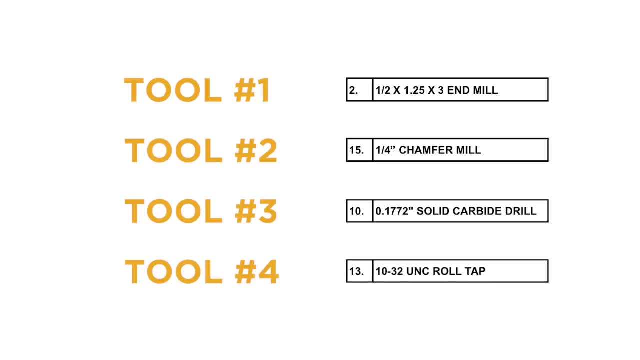 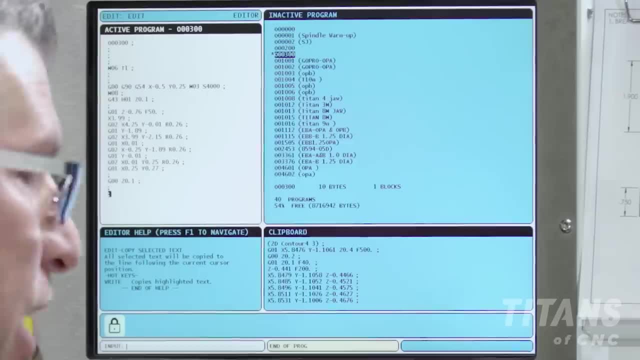 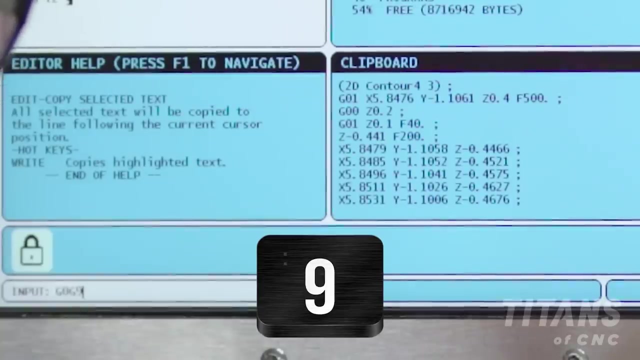 going to go. tool one, tool two, tool three, tool four, All right, So tool two is the chamfer mill, where we're spotting where the drill is actually going to drill for that tap. So let's go grab tool number two, So M6T2.. Boom, So let's go to location. The first hole we'll do is at 0.150 and 0.150.. So 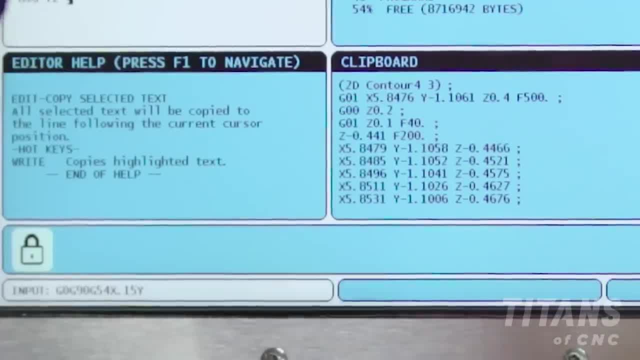 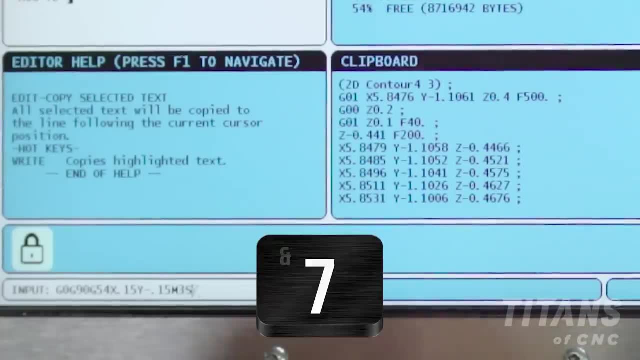 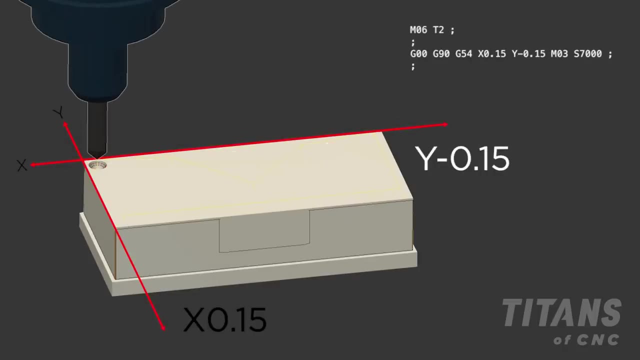 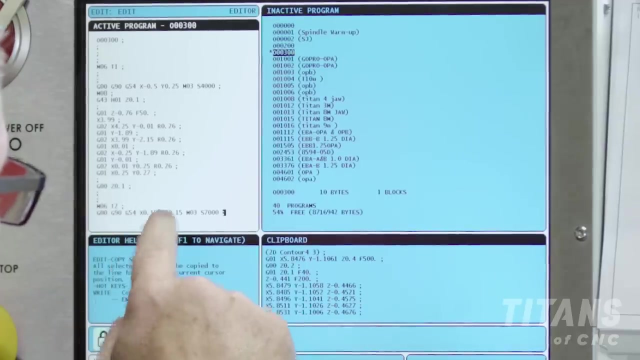 x.15,, y-.15, m three spindle. we'll say 7,000, end the block and we go to location Rapid movement. absolute positioning to the G54 fixture to my x and y location to m three. 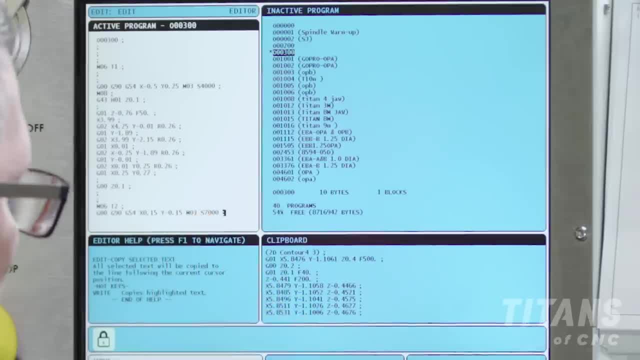 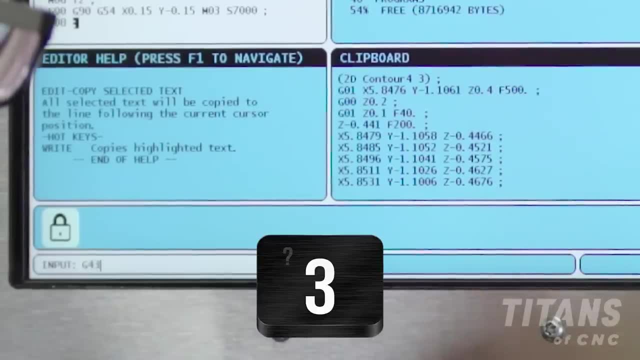 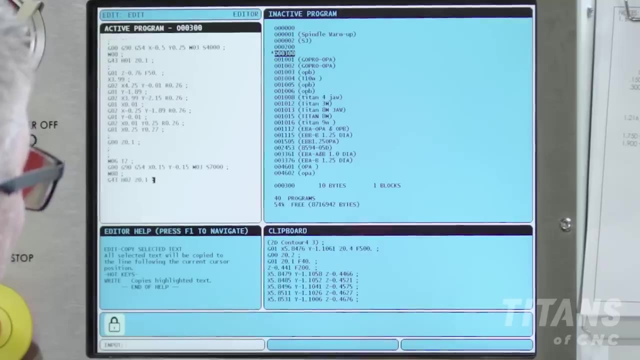 turn the spindle on to 7,000 RPM pms. let's turn the coolant on. let's go grab our tool. height offset g43 h2 z, 0.1. end the block boom. all right. so now i'm going to show you something different than milling. this is a can. 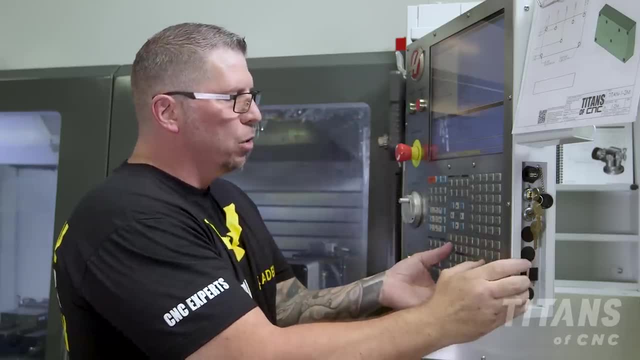 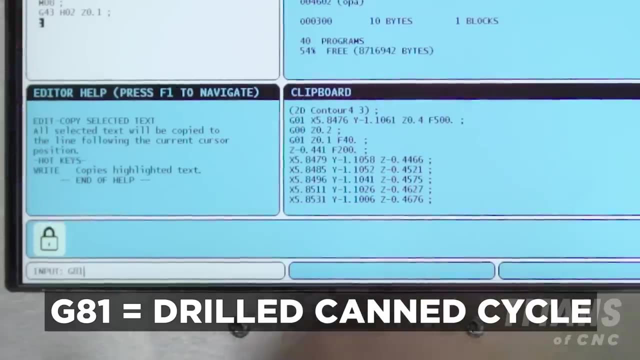 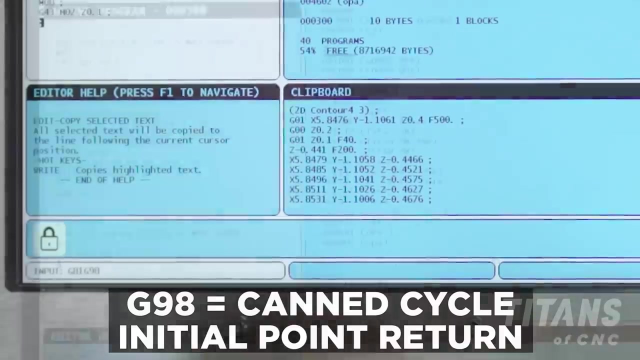 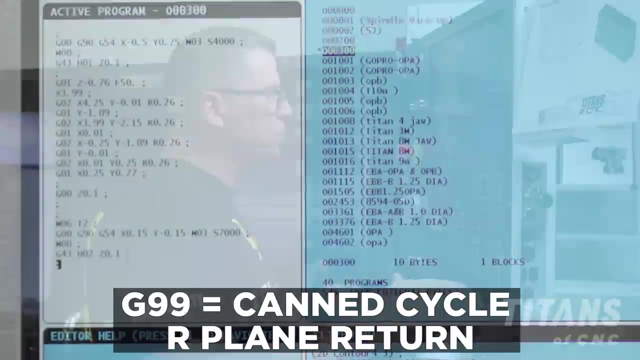 cycle for a drill program. so we're going to go g81 drill with no peck right, just come down, boom, all right. g98 when you raise back up. when the tool raises back up, it would go to our initial plane, which would be on the g43 line. if i had a g99, it would go to our rapid plane. in this case they're. 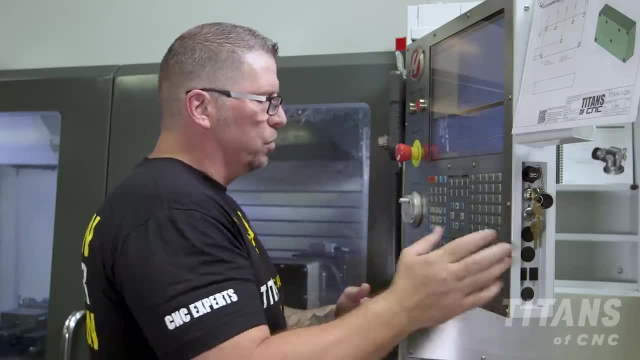 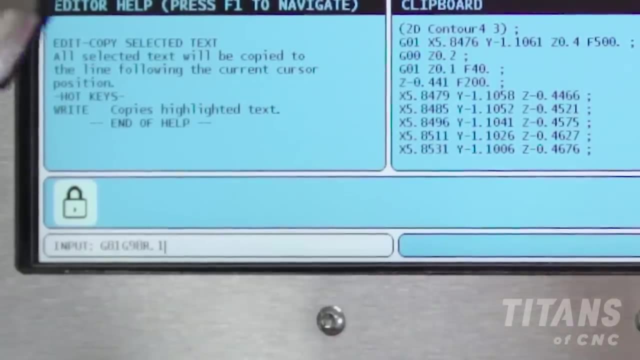 pretty much both the same, because we went z 0.1. so next one is r, which is our rapid plane, boom, boom. then we're going to go depth, so it's a 90 degree included angle. so we're going to go depth, so it's a 90 degree included angle. and then we're going to go. 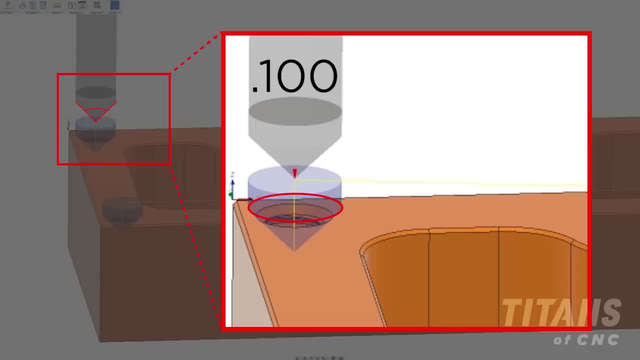 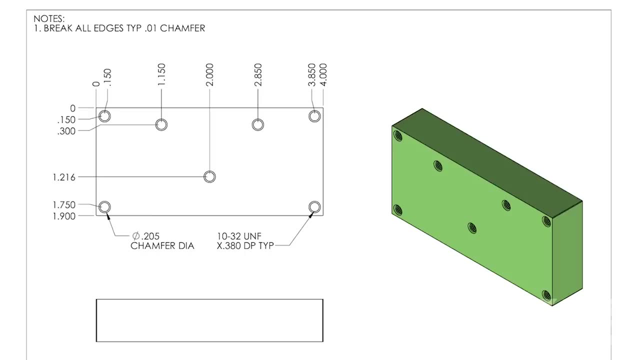 so if i go a hundred thousandths deep, that means it makes that diameter twice as big. so that would be 200 for a 1032 thread. we're actually going to build a chamfer. that's about 0.205, so i'm going to. 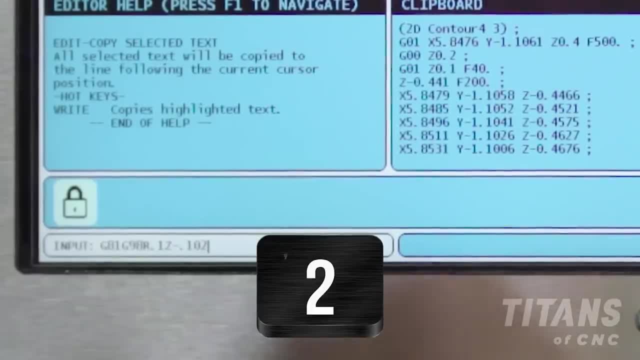 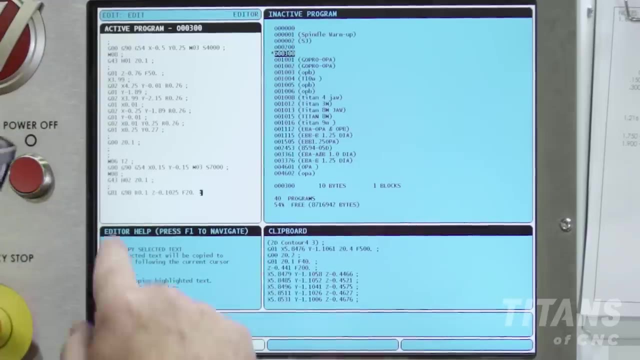 go negative 0.1025, and then i'm going to hit feed rate, i'm going to hit 20 point and i'm going to hit end the block. and there you go. end the block, and there you go. so now you have your drill program. when you raise back up, go to your. 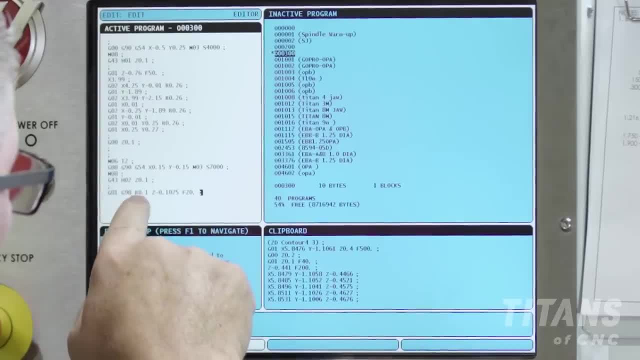 so now you have your drill program. when you raise back up, go to your rapid plane. r1 is your rapid plane. z negative 1025 is how deep we're going and we're feeding at 20 point, which is 20 inches per minute. the cool thing about rapid is, if you were in a pocket and you were way down here, you could actually 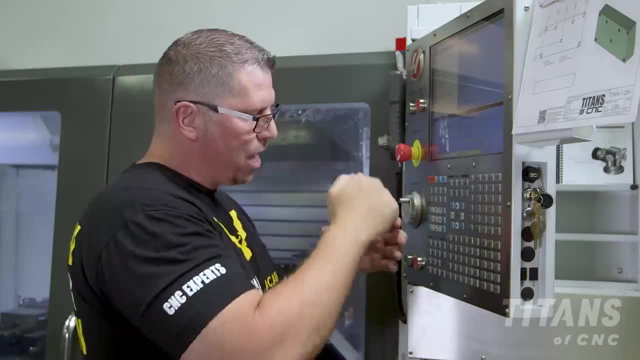 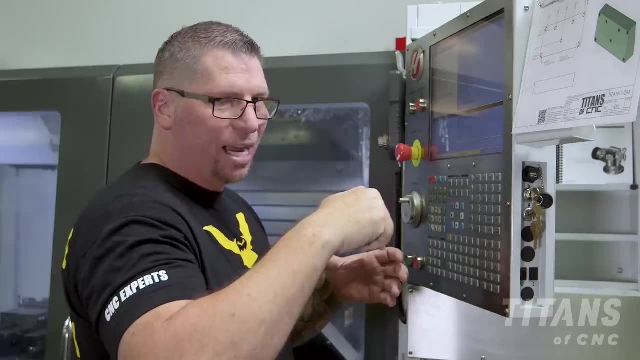 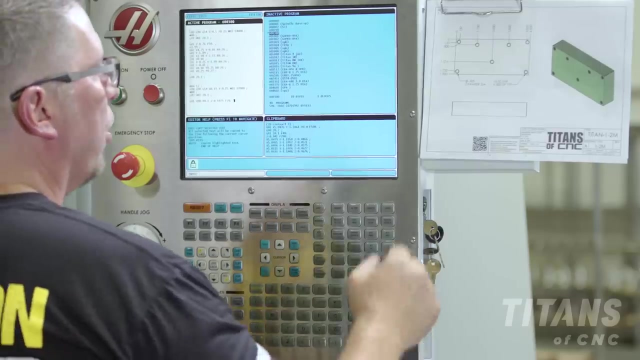 instead of raising all the way up, you could keep your r down and actually stay down and be like boom boom, boom boom and then raise it up before you hit the wall. right so, but that's advanced programming. right now, you want to stay above z and not mess with it. okay, so, all right, so we're going to walk. 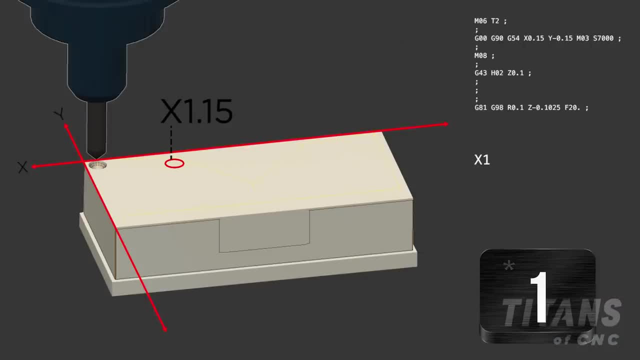 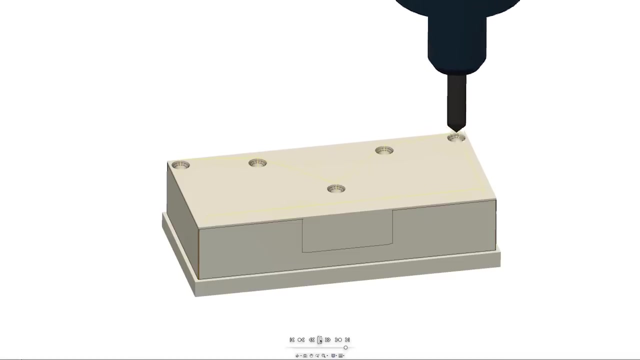 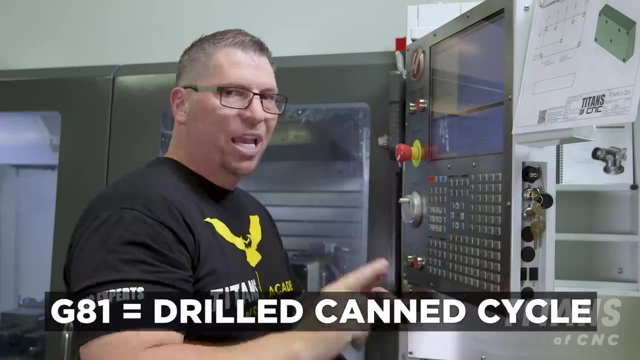 right around here. so we're going to go x, 1.15, y negative, point three. boom, that's our next location. a can cycle is modal. that means that you can go location to location, location. it'll keep drilling the exact drilled hole, the g81, at that depth, until you cancel it. and when you cancel it, that would be. 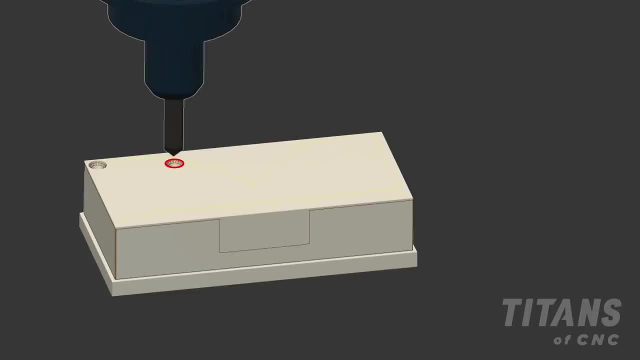 a g80 and i'll show you. so pole location is right there, so we're going to go. next, the third hole is two point and then y negative. one point, two, one, six, boom, i'm going to hit, end the block. boom, i'm going to go back up here. i'm going to say x, 2.85, y negative. 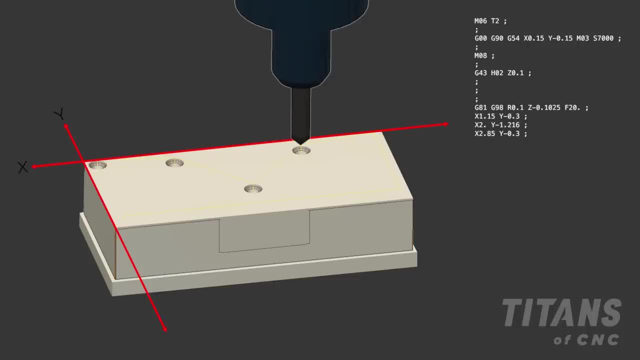 point three: boom, i'm gonna hit x three. point eight: five. y negative. point one: five, that's that one. i'm gonna boom, i'm gonna drop down. my x is going to drop down, my y is going to drop down, my x is going to stay the same. so i'm just going to hit y negative 1.75. i'm going to enter. now, i'm going. 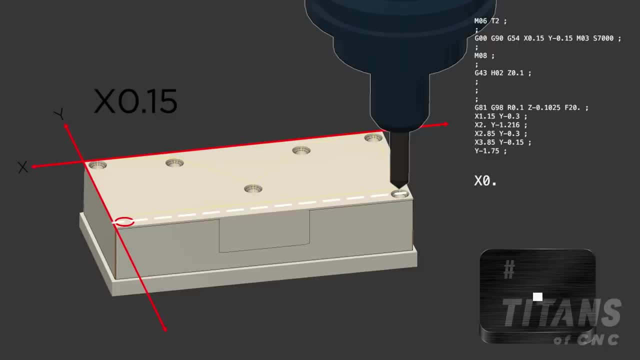 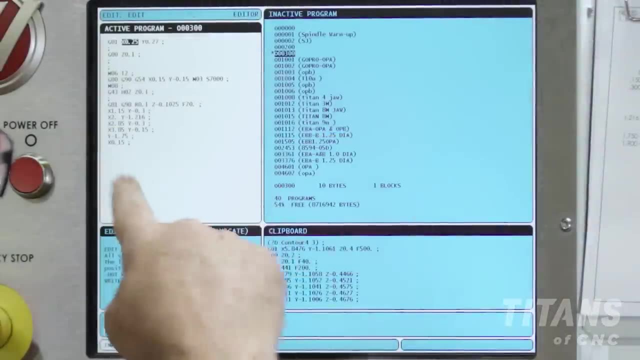 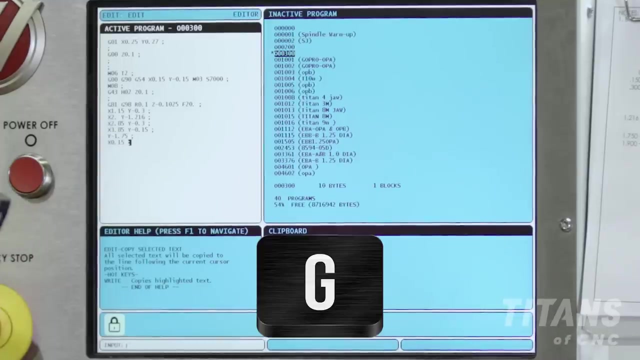 over here. so i'm at x point. one, five, i'm gonna enter now i have all my drilled holes right here. boom, boom, boom, boom. there's one, two, three, four, five, six, seven. one, two, three, four, five, six, seven. that all looks good. so now i'm going to end it with a g80. so right here i'm going to say g80. 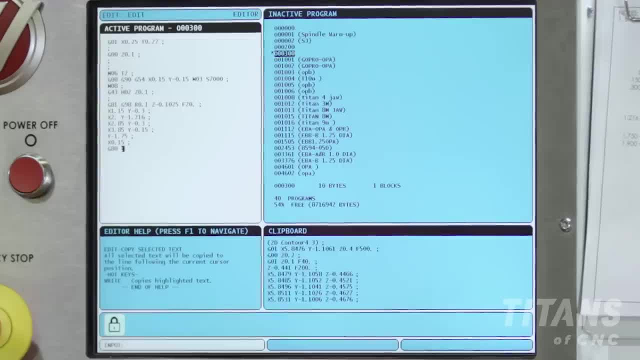 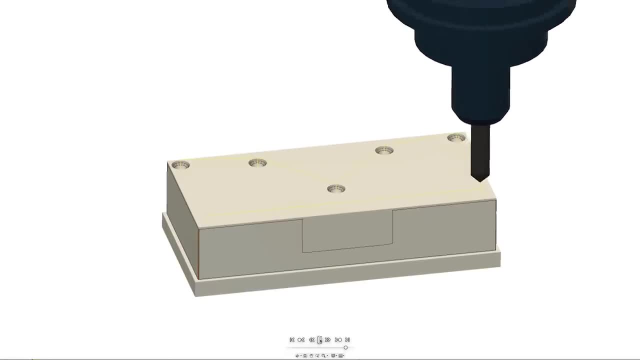 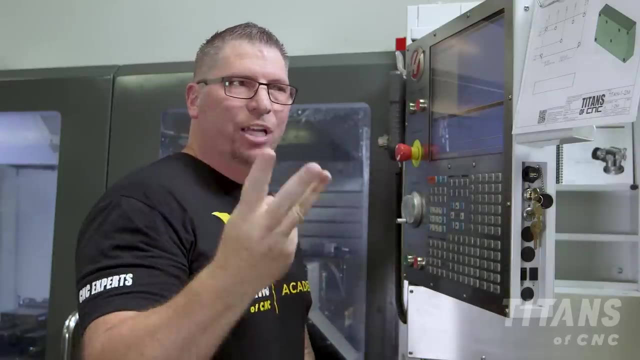 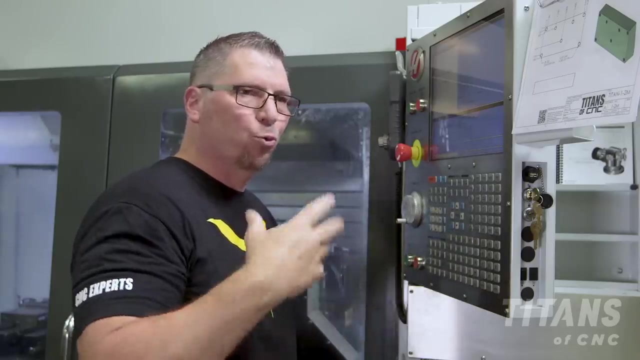 cancel can cycle. boom, it's cancelled. all right, and then now that's done. now here's the trick. so i just gave you a drilled program and i have three different tools that are doing similar can cycles. right, the drill program is the can cycled and i have three tools that are. 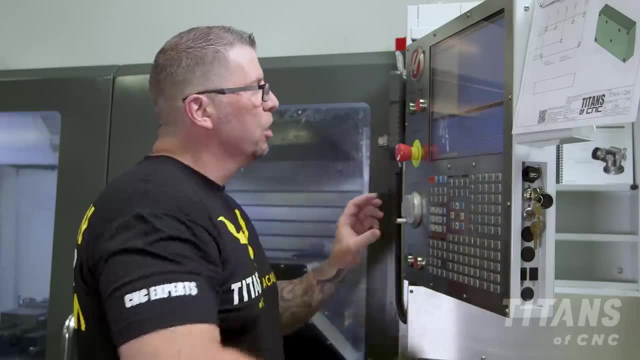 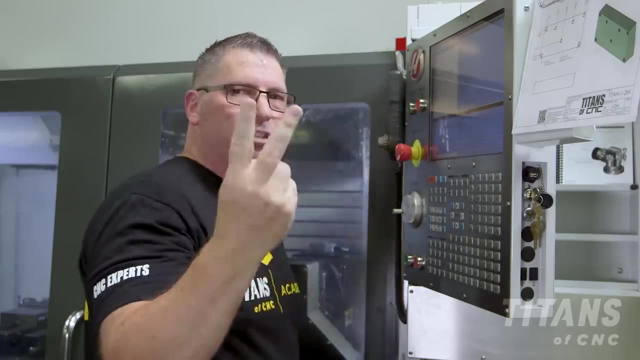 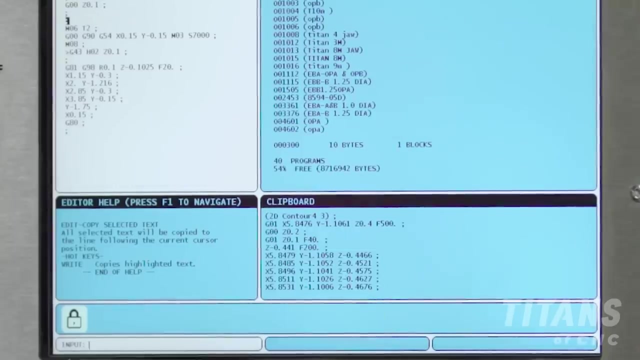 doing basically the same thing with the same motion. okay, so watch, i'm just gonna come down here right above where i wanna start, and i'm just gonna copy it and i'm gonna paste it two times because most of the information is gonna stay the same. so i'm gonna hit f2, i'm gonna scroll down. 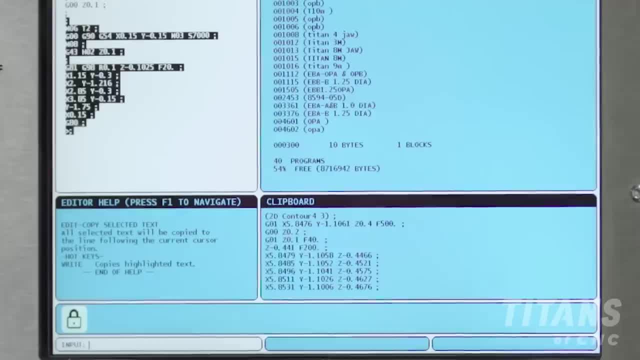 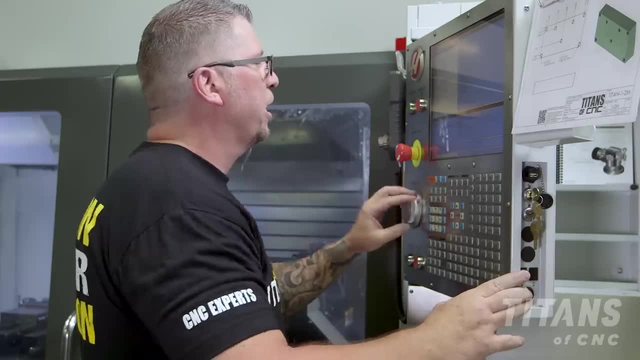 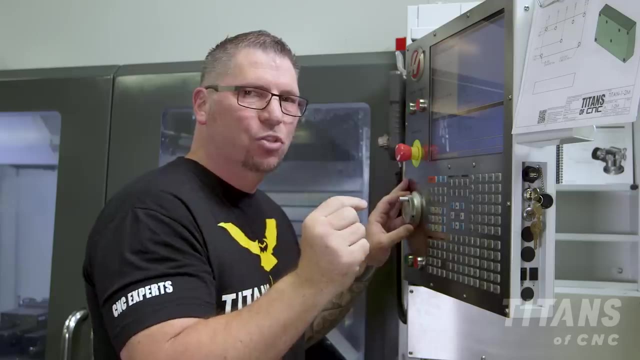 boom, i'm gonna hit it one again and again. now i have three of them right here, okay, and now i simply have to change my t's and my h's. you always want to make sure that your t and your h are exactly the same, otherwise you can crash this machine. 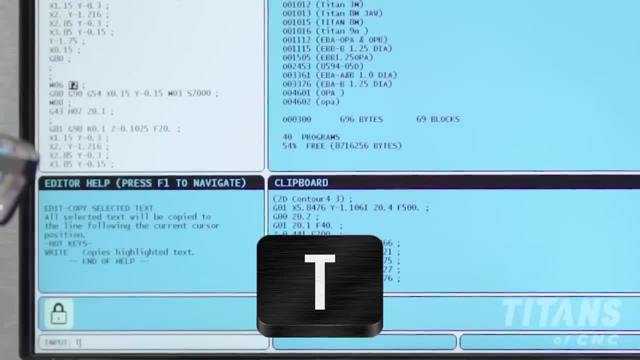 so this one is now going to be, this one's going to be tool three. i'm gonna hit that guy. i'm gonna hit h3, h3. i'm gonna hit that guy. i'm gonna look at it. now we're drilling right, so let's change. 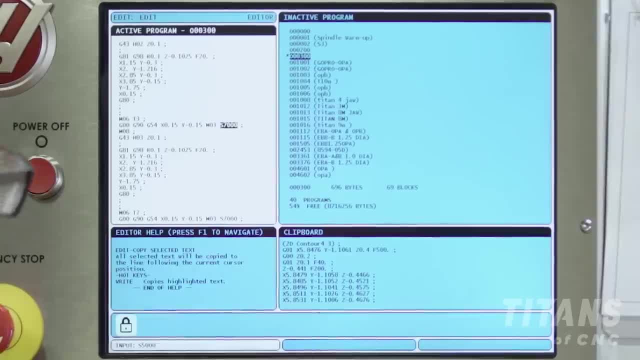 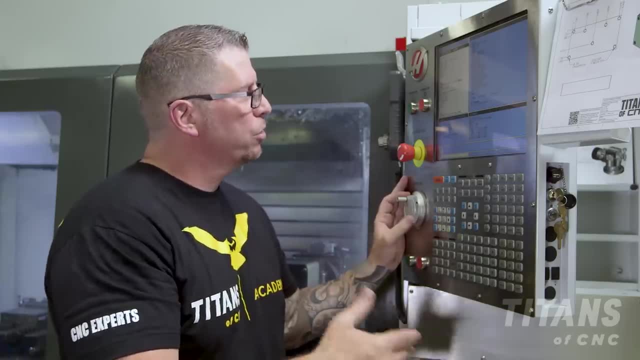 the rpms a little bit. i'm gonna go five thousand, hit that bad boy right there. we're using a kind of metal drill so you can actually go three times diameter, so it's a pretty awesome drill. just to be safe, because i'm teaching gnm code. 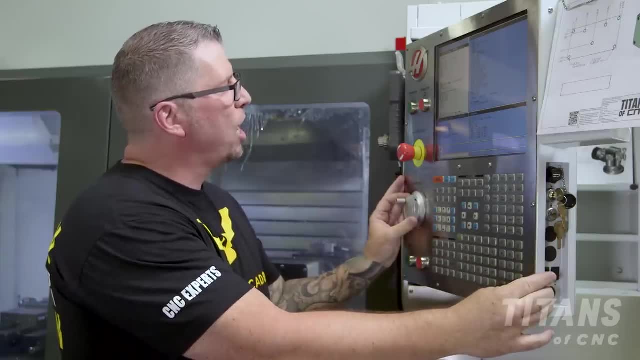 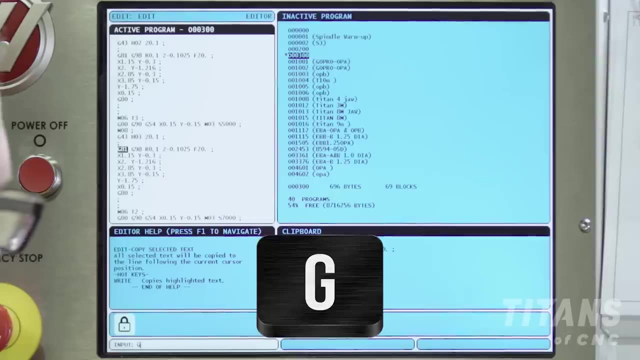 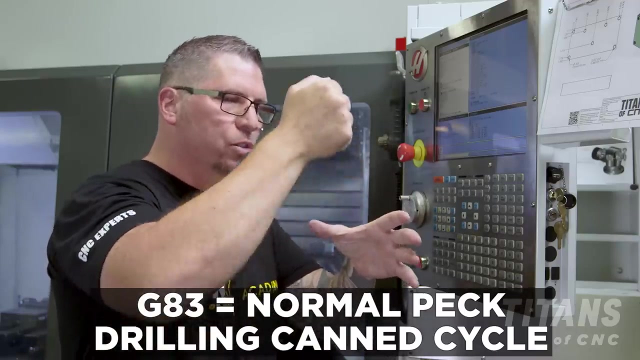 i'm actually going to stay a little bit shy. so what i'm talking about is this: g1 is one movement drilling straight down and coming out. g83 is a drill movement with a peck, so as you come down you can say: go a hundred thousand, 200, 000, 300, 000, so you can break that chip and get the chip out. 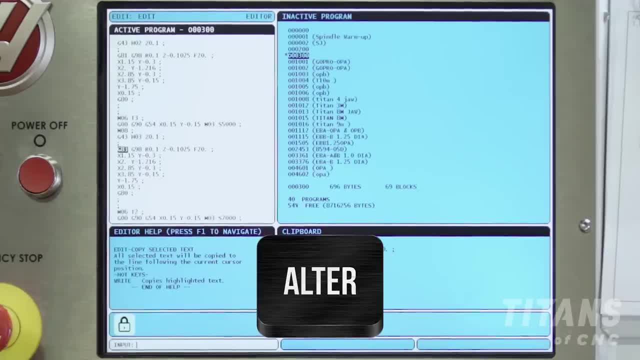 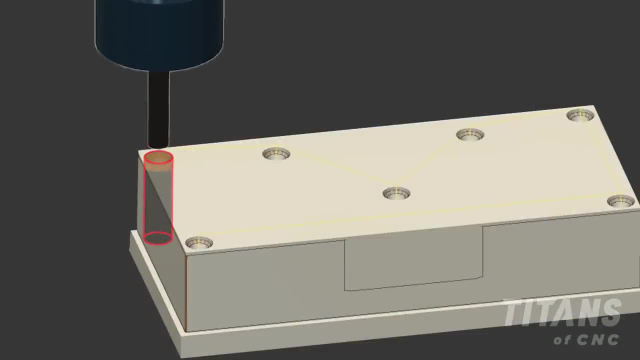 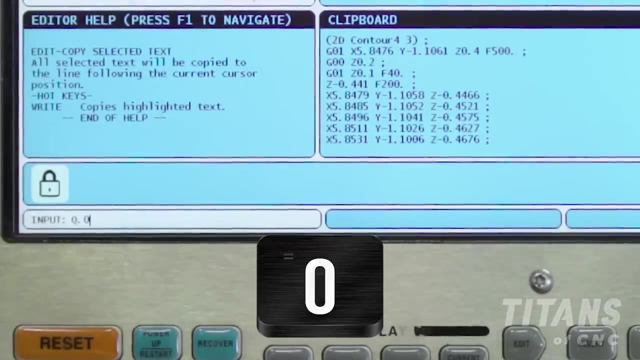 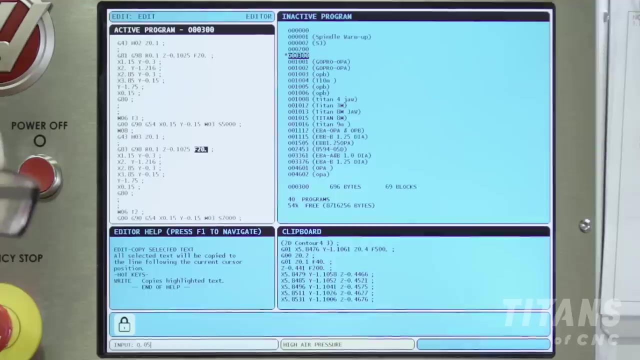 okay, so we're gonna hit g83 and now i'm gonna leave everything the same, but i'm gonna add a q as the size of the peck. so boom, boom, boom. so we're gonna do a q of q point zero, 50, just for safety. this kind of metal drill can kill it. i just want to be safe, all right, and we're just. 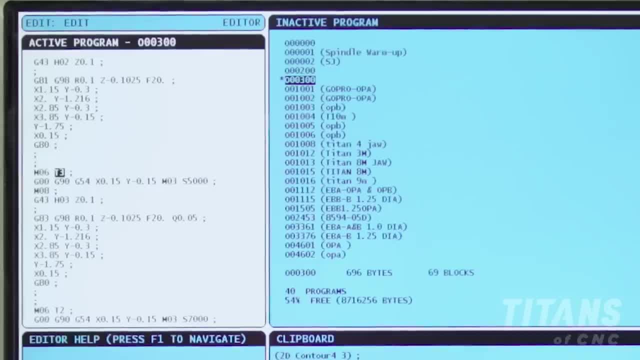 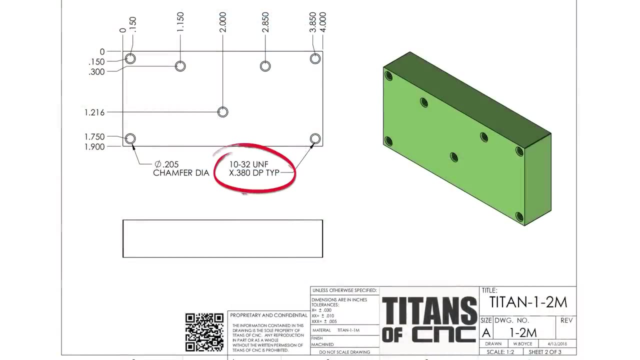 going to insert this guy now, t3, h3, although always double checking: boom boom, g83, boom boom. but how deep am i going to go? so i come over here. it says 380, so i'm going to go 580, so i'll go z negative. 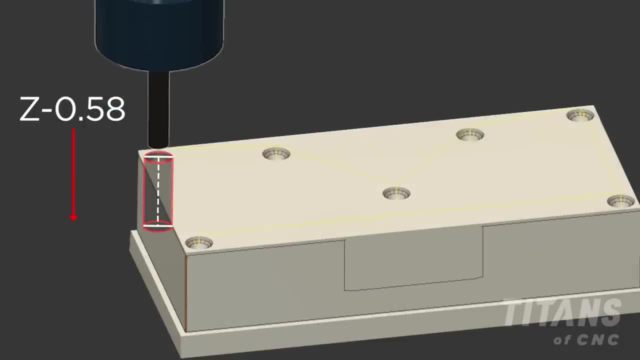 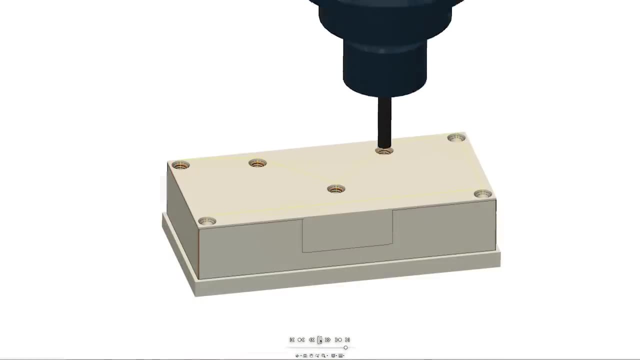 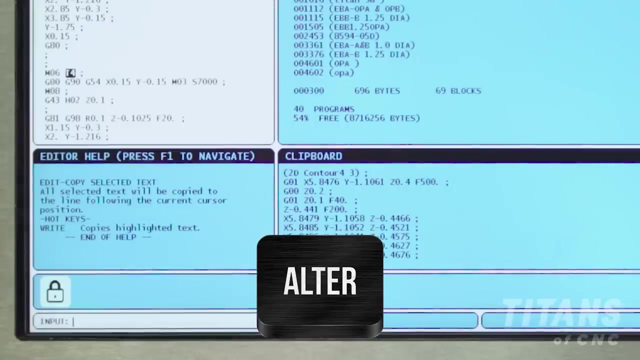 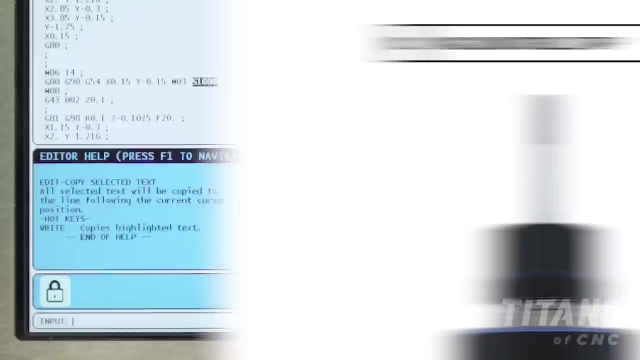 0.58. so i go deep now and it's going to pack 50 thousandths at a time. so now i come down here, i hit t4 right there. i'm gonna hit one thousand because now we're tapping. okay, so tool 4 is a 1032 roll tap. okay, we got cooling in the machines. 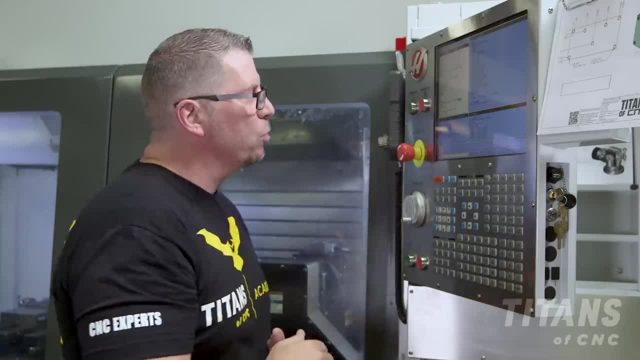 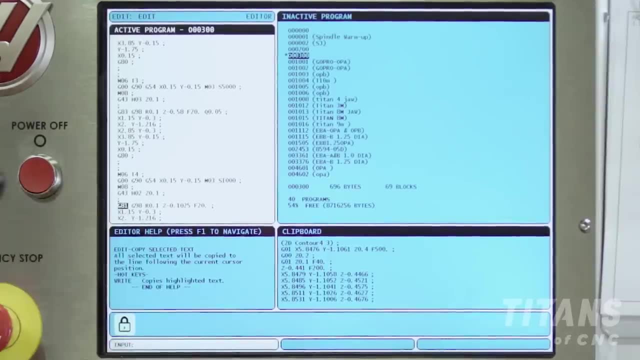 the roll taps, like the heat. i'm going to run it at a thousand rpms. i'm going to leave everything the same, but i'm going to change this to the tapping cycle and that's a g84. so we're going to go g84 foam. we do not want it to hit the bottom. so i'm going to say a hundred thousand four hundred. 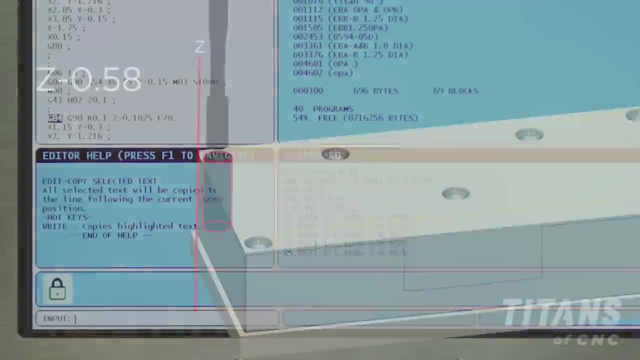 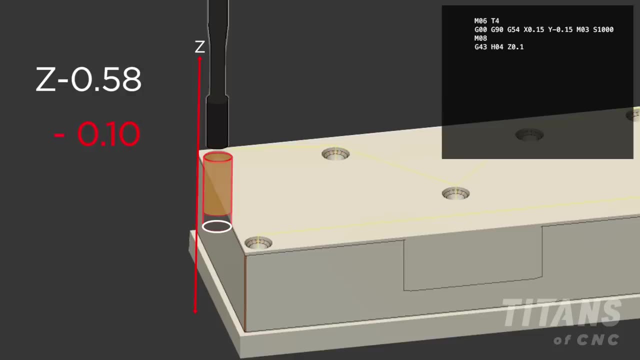 thousand four and that's a g84. so we're gonna go g84 foam. we do not want it to hit the bottom. so i'm going to say z negative 0.48, which is a hundred thousandths shy of the depth that the drill went. 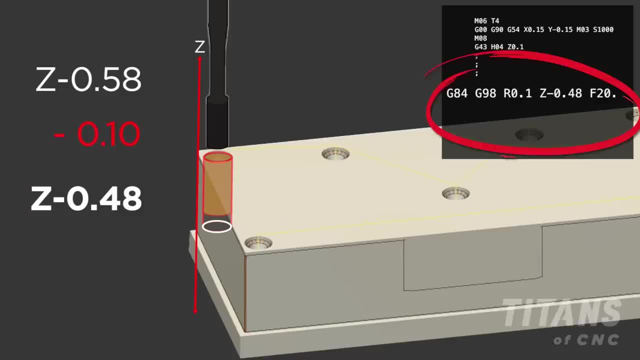 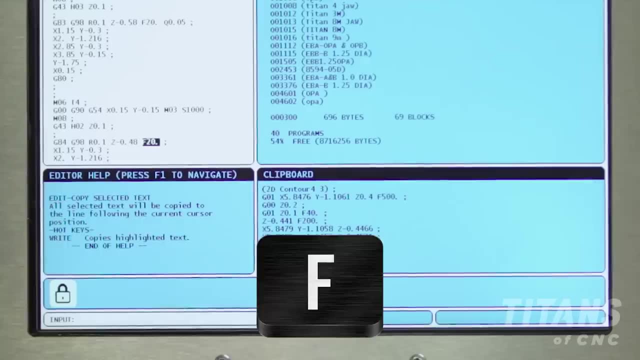 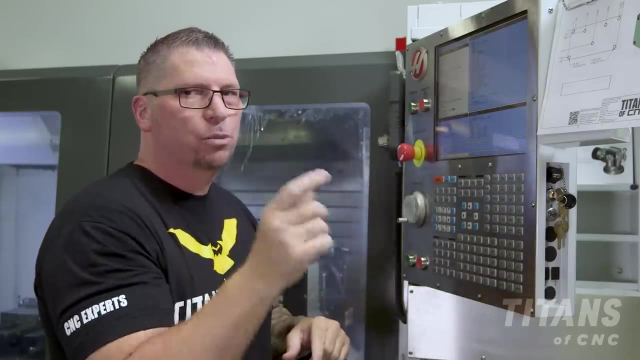 down, boom and over. here. i'm going to put the exact feed rate when you're tapping. there's a calculation, it has to be perfect. so this is feed 3: 1.25, because i'm a thousand rpms and i have 32 threads per inch. so i'm going to put the exact feed rate when you're tapping. so this is feed 3: 1.25. 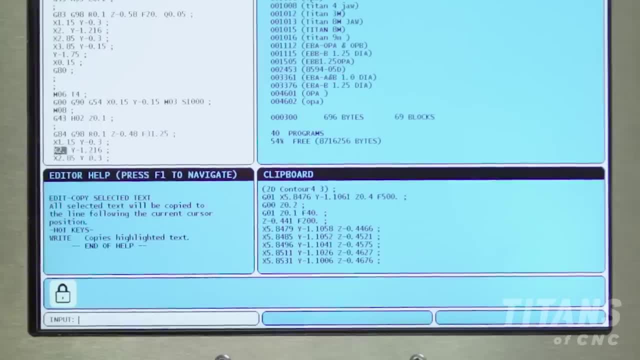 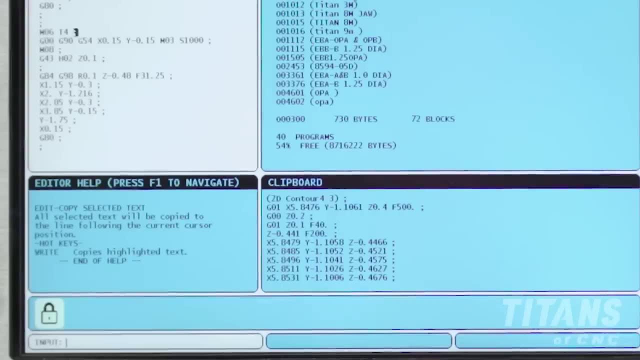 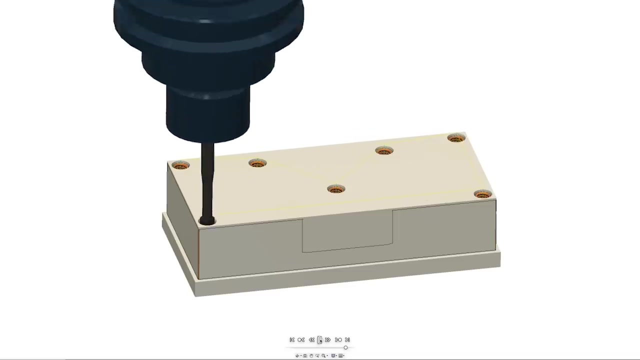 on that thread. so i hit that guy right there. i said i needed my h and my t to be identical- t4, h2. so let's go h4, foam- and we are perfect. so now we have tool 1, tool 2, tool 3, tool 4, all dialed. now we just have to finish it up, right. 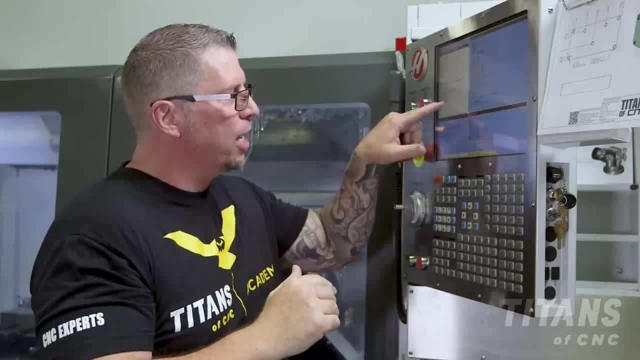 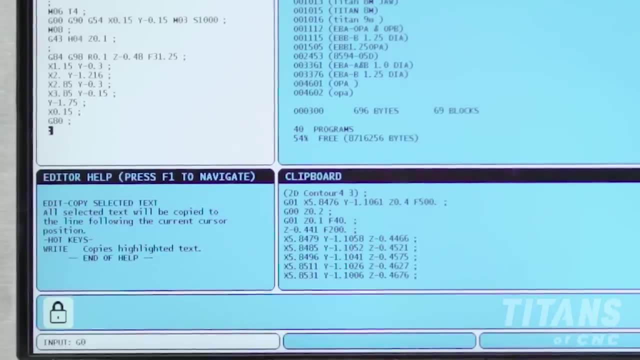 there, okay, and i'm gonna go ahead and hit the h height now, because i'm thinking about my height offset for tool 4 right now. okay, but i want to send it back home, so all i'm going to do is hit g0- rapid movement, the height offset, the g43 line. let's cancel that. that's a g49, boom, g49. 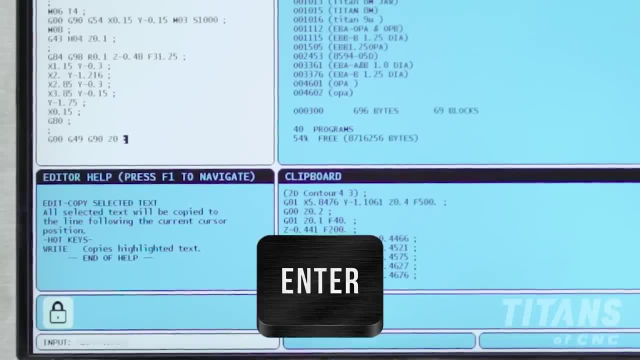 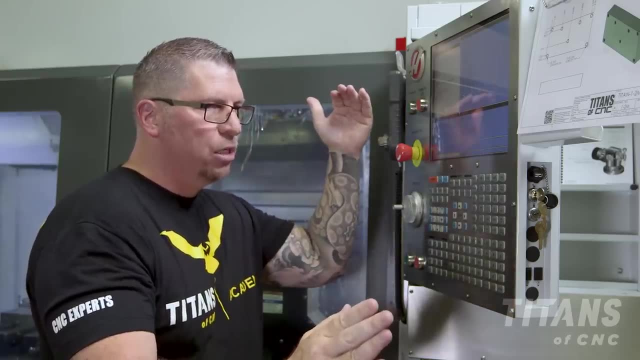 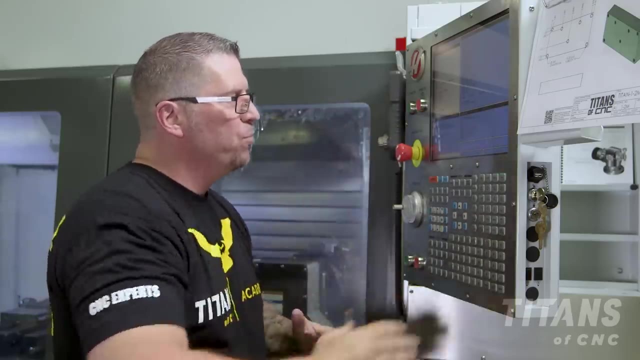 all right. and then g9, zero, g90, absolute positioning, z0. i'm gonna enter that base vídeo here on the. that basically cancels the height offset. Now the machine's reading its home position. You say Z, zero. it just goes home, which is top of the movement, okay. 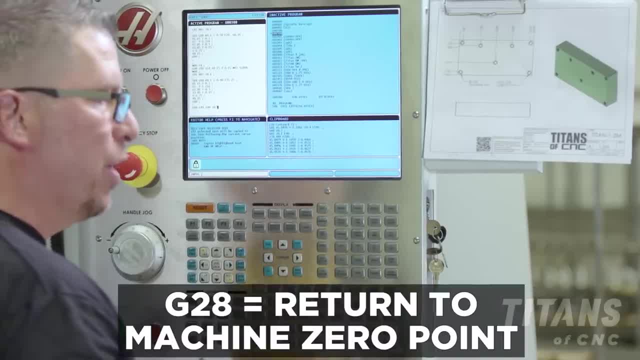 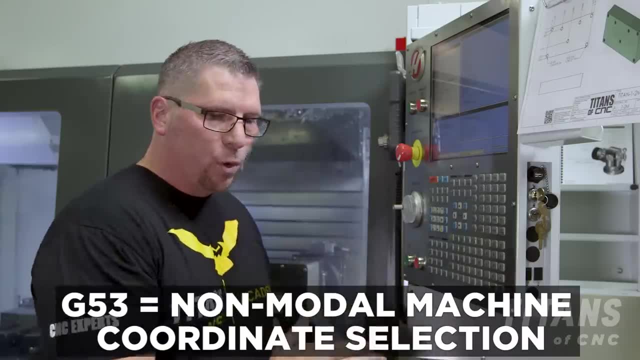 Now there's two ways to home the machine. You can do a G28 or a G53.. I'm actually gonna use a G53 because it allows me to put an X movement and position my table where I want it. So if I wanted my table moved, 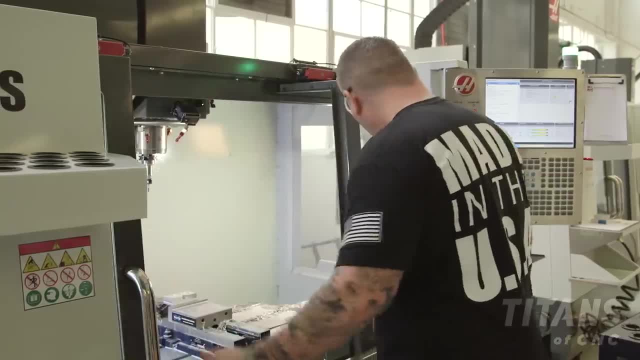 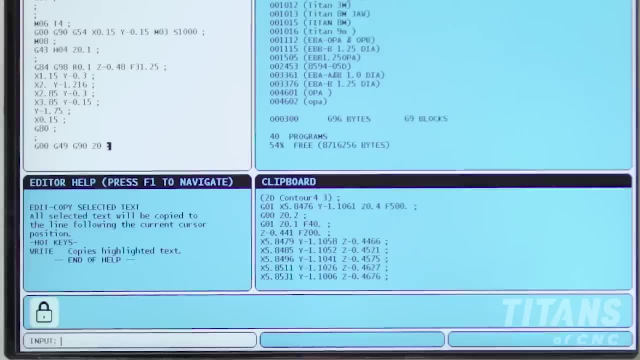 so I could actually open the doors and have a vice at a specific spot. I can actually change my X, so the table moves perfectly into position. So I'm gonna say G53, X negative 30 inches, Y zero enter, and then I'm just gonna hit M30,. 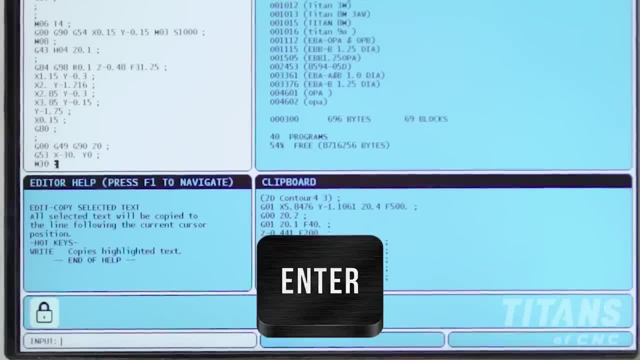 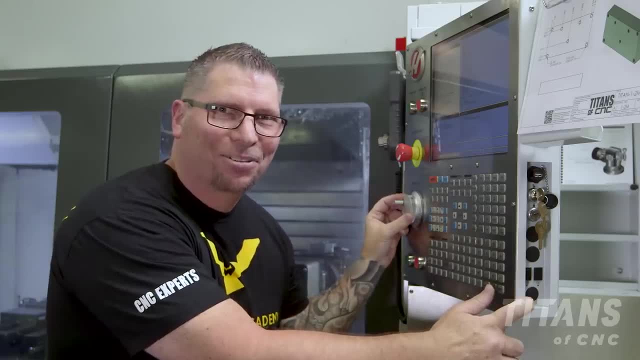 shut it down, end the program. boom, and that's your program right there. All right, But did it work? I don't know, Like we were going pretty fast, So how do we actually double check it? Okay, we're in here. 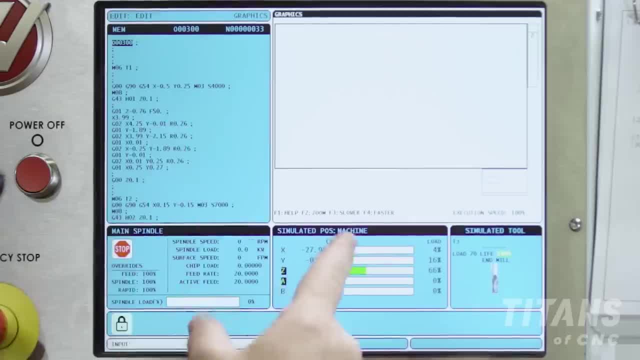 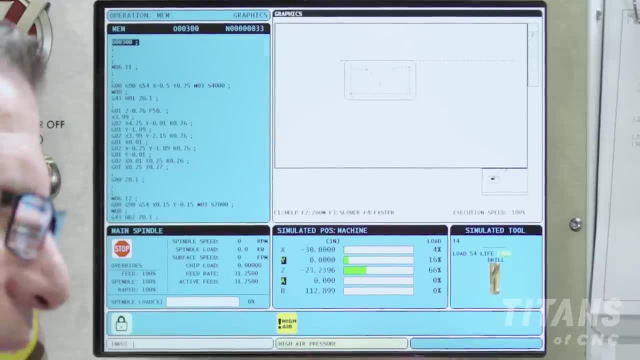 We're gonna hit setting graph one time. Just hit the start button, Boom, it goes around, goes around, goes around. Oh man, it looks good, all right. So what if I can't really see what's going on? 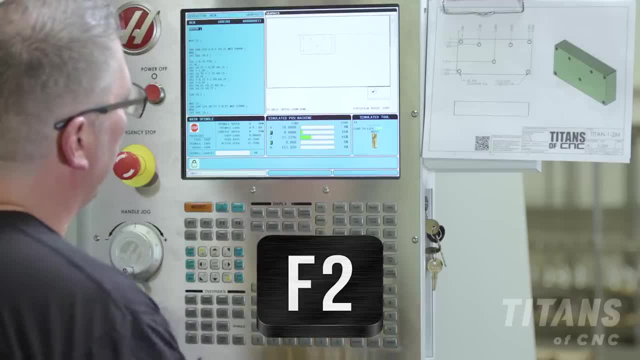 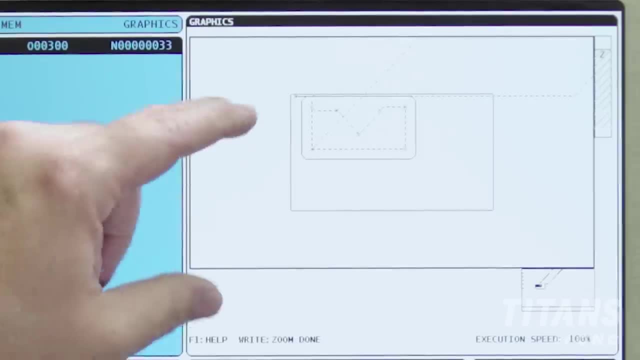 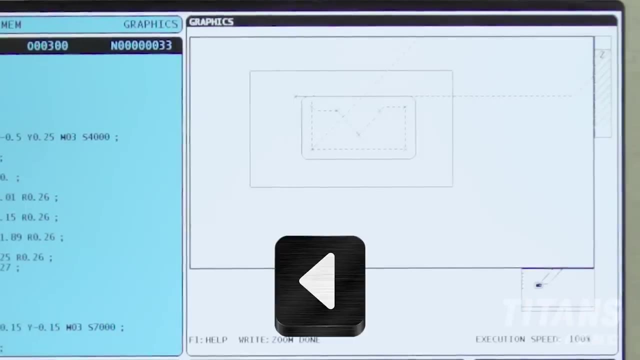 Okay, one thing that I can do is I can actually hit F2 right here. That'll zoom it, and then I can just basically come down and I can actually page. So see that little square right there That represents the entire block right here. So I'm going to come up, I'm going to come over, I'm going to look at my part. 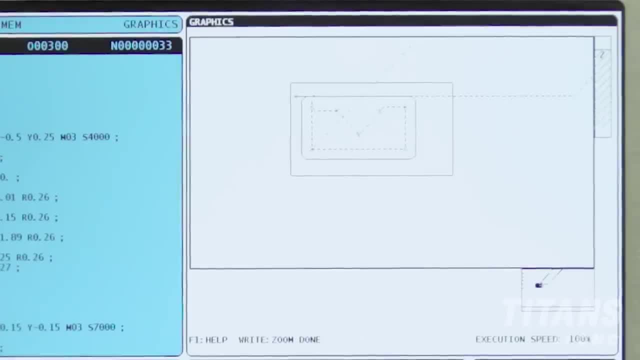 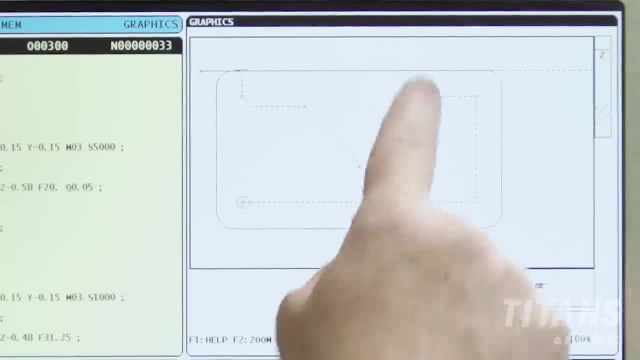 I'm going to actually just see if I can get a little bit closer, See that. Then I'm going to hit enter. Then, if I do it again, oh, I can see every single radius, every single radius, Boom, boom, boom, boom, boom, boom, boom. So I'm looking at my part, I'm looking at the outside. 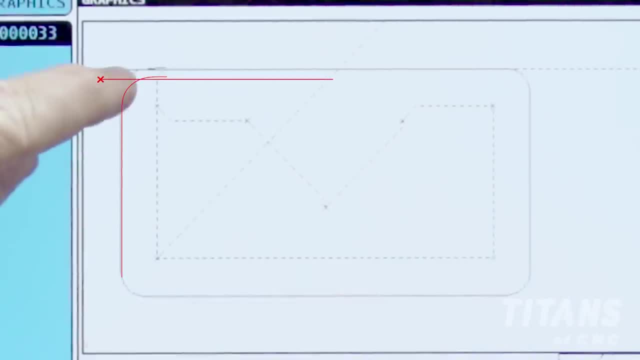 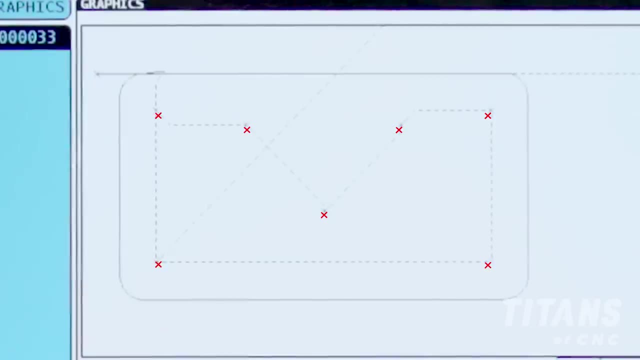